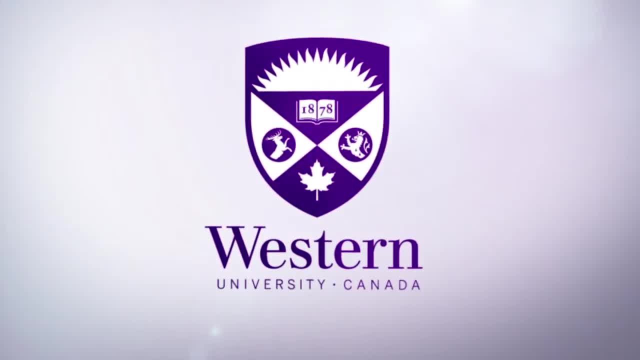 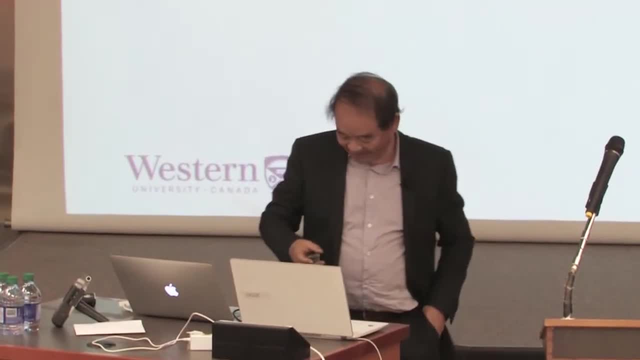 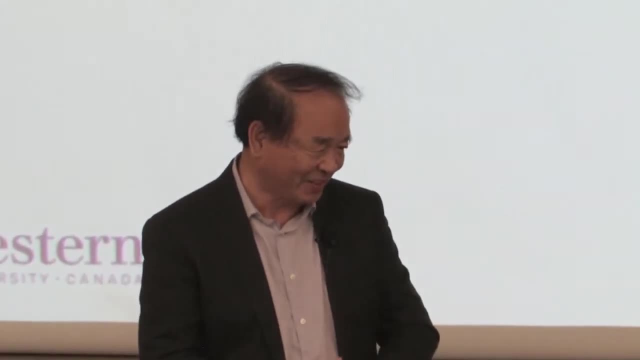 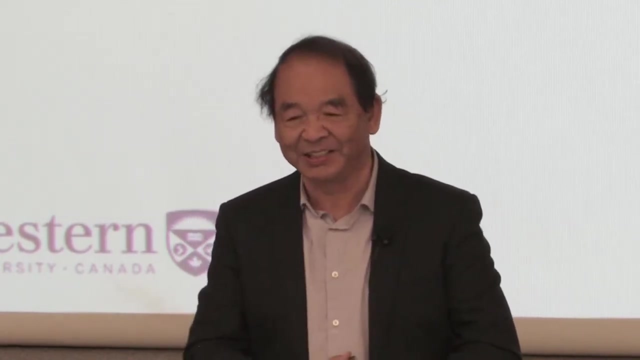 Thank you, Janice. I'd also like to congratulate Mary and Jeff for the award, and I really learned an awful lot from your talks. Before I start, I'd like to thank my wife and my daughter. They are in the audience Without their support and understanding over the years. 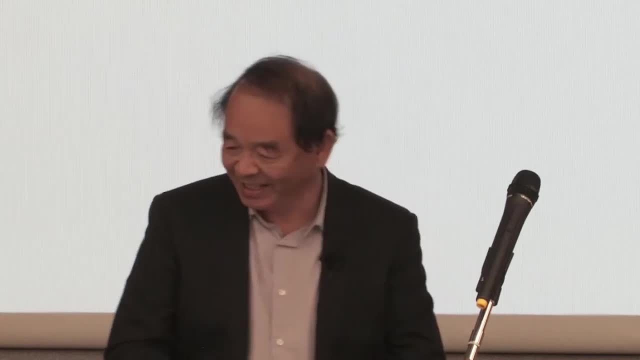 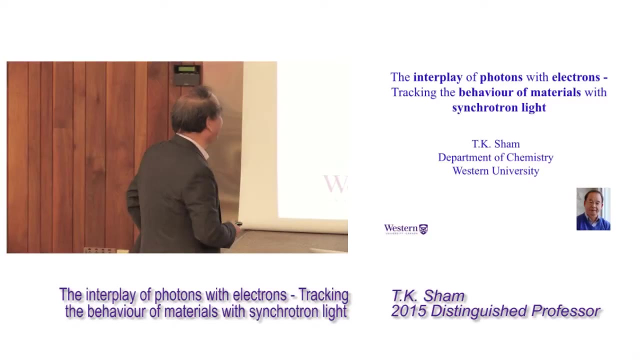 I would not have been able to have so much fun with the singletron. That's what I'm going to talk about. Okay, let me begin with the peculiar properties of light. You know, when you switch on, when you go into the room, you have light. So this is some other definition. 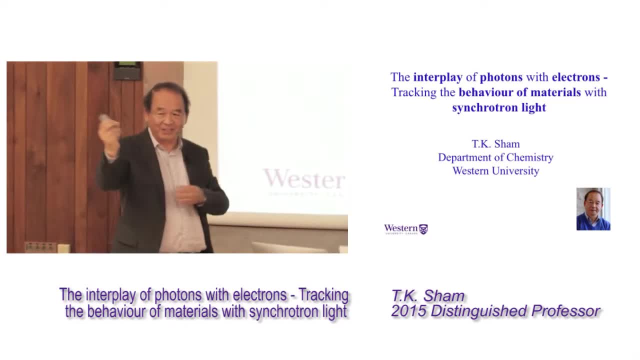 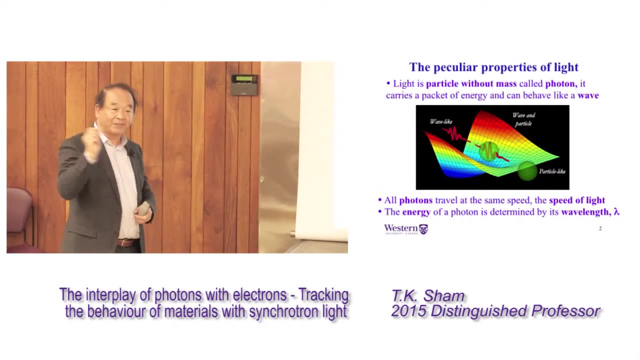 Now, light is in fact a particle When you are looking at something actually on the floor, the photons are coming in the eyes right, And they have a name called photon And it actually carries some energy, okay, And it also behaves like a wave And that. 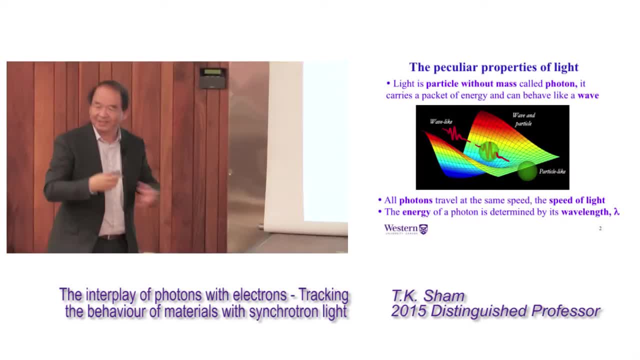 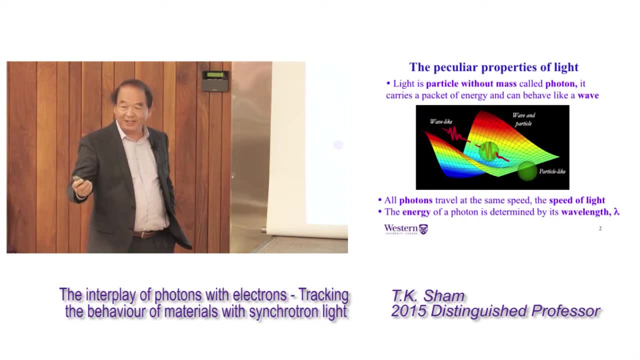 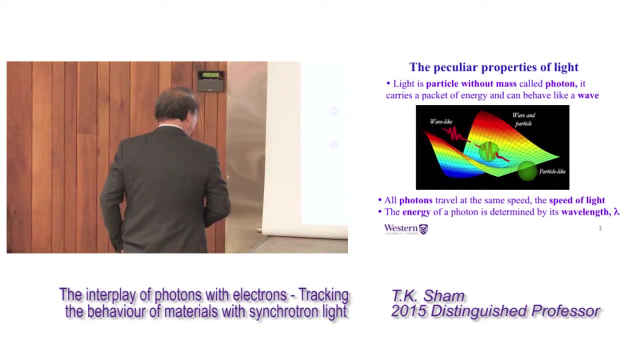 is really the dilemma of nature, something which is kind of variable. Now, the other property of light is that all the photons carry energy, and the energy is determined by its wavelength, right By its wavelength. Now, strangely enough, light is not a particle. It's a particle. It's a particle of light. 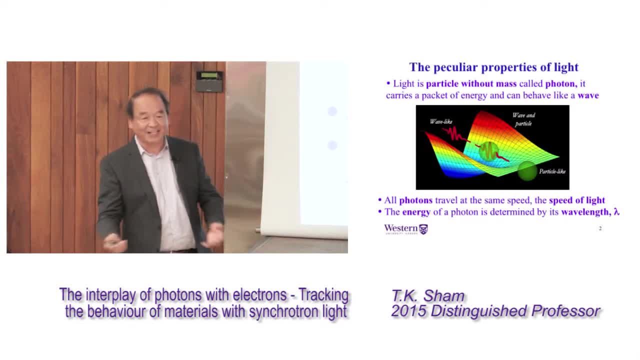 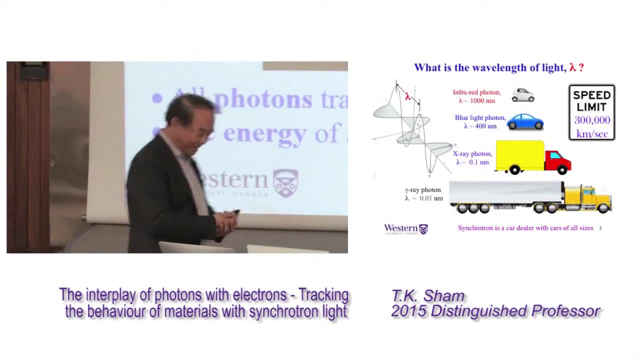 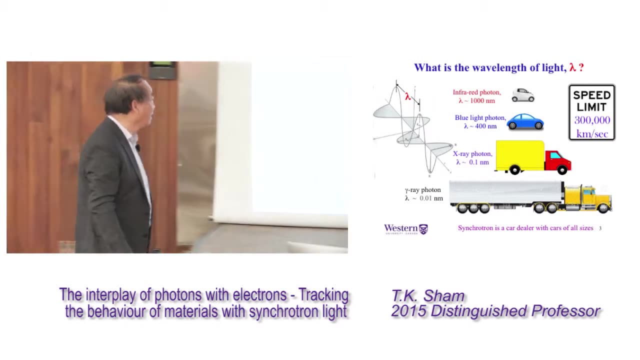 Now, all the photons travel at the same speed. whether it carries a lot of energy or carries very little energy, they are as fast as each other. okay, So these are the really peculiar properties of light or photons. So what is the wavelength, right? I mean, it's kind of. 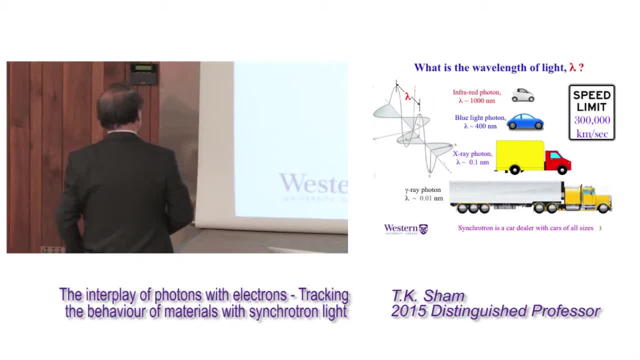 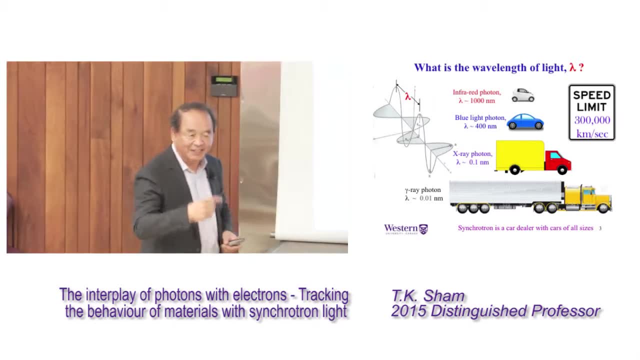 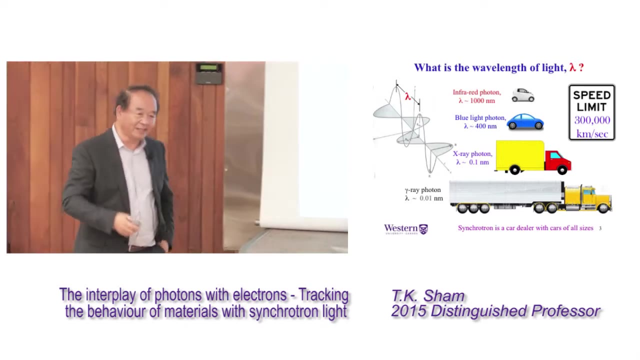 a benchmark of a photon. Let's imagine a photon propagating in space travel. Let's imagine a photon propagating in a wave, such as a sine wave of oscillating electromagnetic field as described by Maxwell. okay, Then the distance it travels at a given interval. 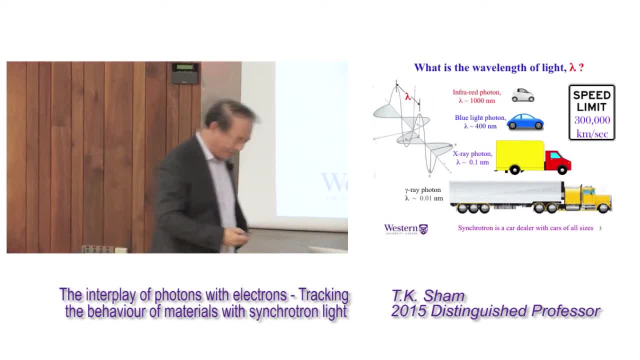 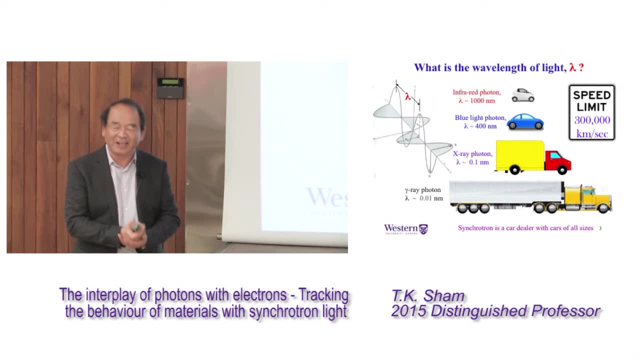 is the wavelength. So that's the wavelength. okay, So now, if you consider an infrared photon as a smart car right, with a wavelength of 1,000 nanometer, Then a blue light photon would have a wavelength of 1,000 nanometer. Then a blue light photon 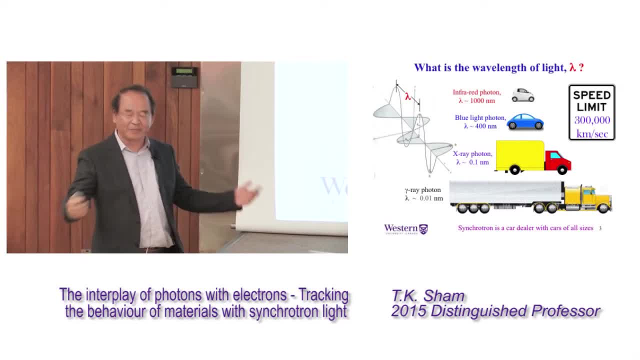 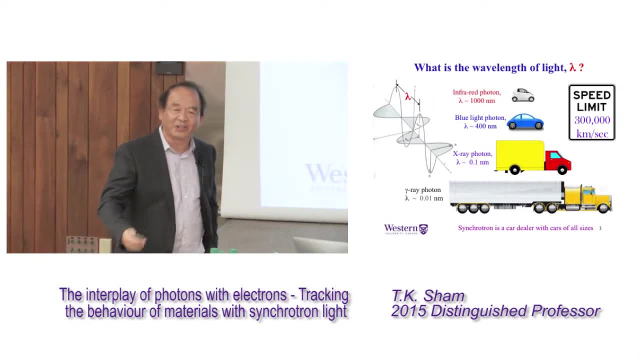 would have a wavelength of 1,000 nanometer, Then a blue light photon would be a sedate right. so a little bigger carries more energy, And if you go to x-ray you have a trough. you have a trough. But if you go to gamma, 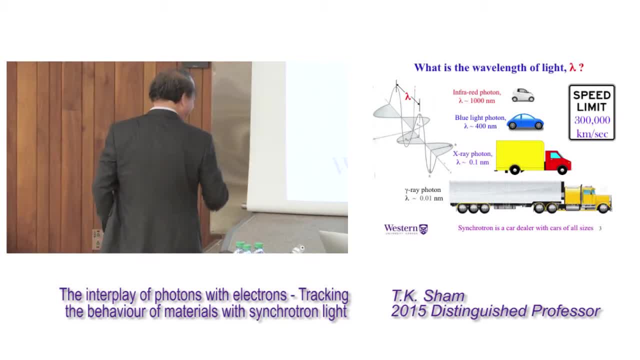 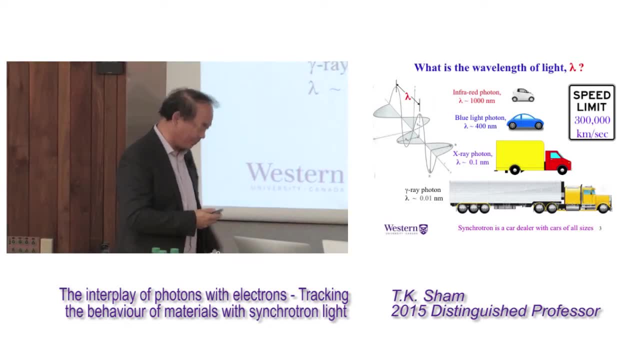 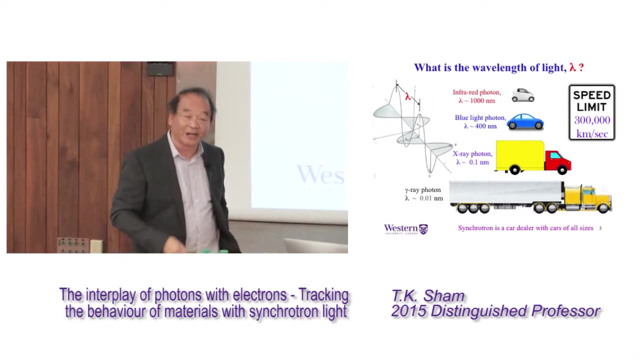 ray, you have a bad trough. So therefore, a single trough can be regarded as just a car dealer, as a car of all sizes. They all travel at the speed of light. Okay, speed limit: 300,000 kilometer per second. They all travel at that speed and that's. 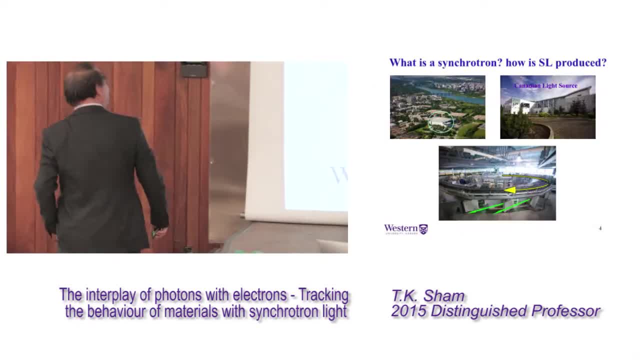 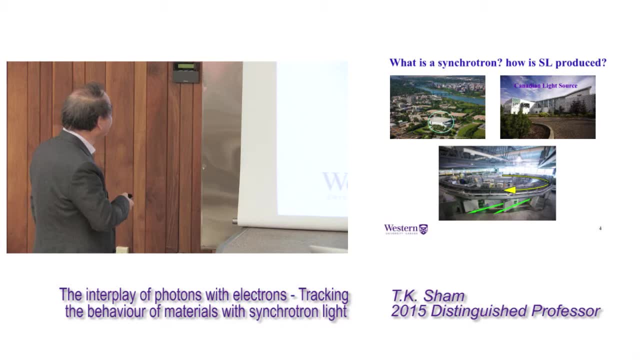 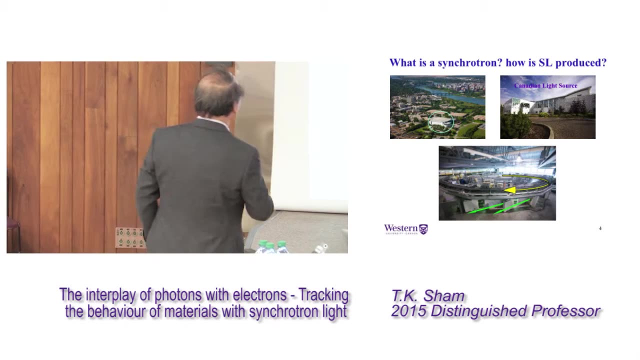 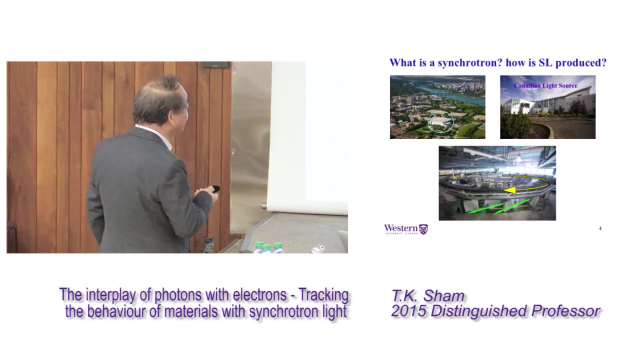 life. Now, what is a single trough? So on the left you can see this is the building that holds the Canadian NISO, the one and only single trough in Canada. It is in Saskatoon. Now on this side you can. this is sort of a ground level view of the building. 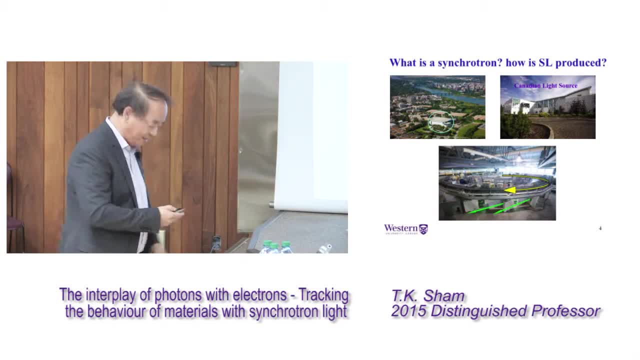 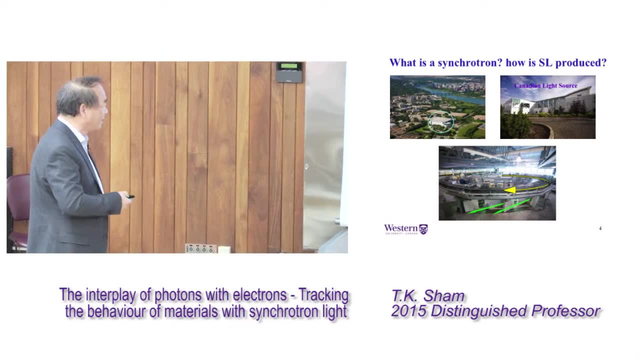 The building is sort of like a stadium. it's very big And inside you can see this is the stadium And inside you can see this is the stadium And inside you can see this is the stadium And you can see this is the elevator, sometimes called the storage room. 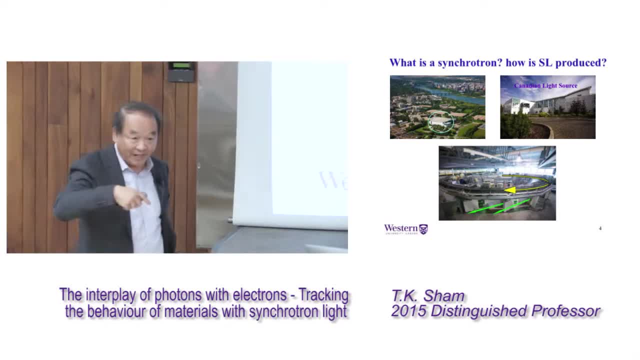 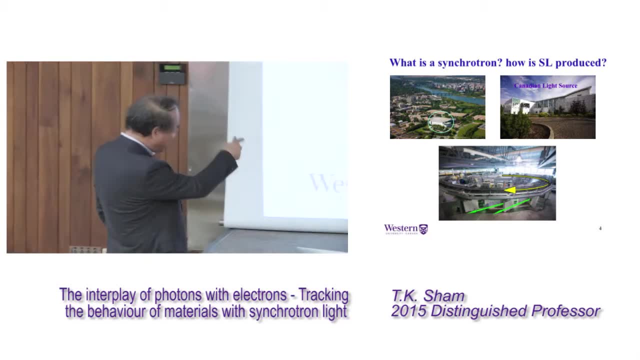 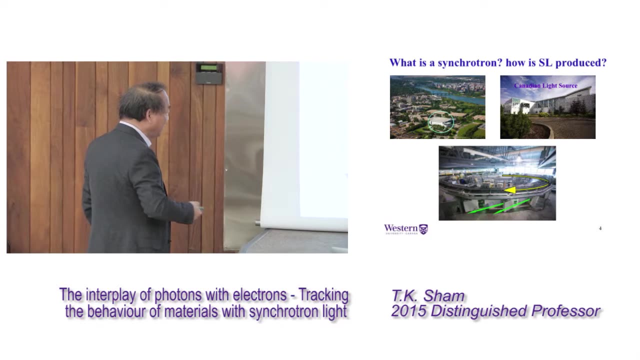 So here electrons are forced to circle Right, They are forced to circle at very high speed, close to the speed of light, And when that happens the electrons bend. in effect they bend by a mallet, and then you can see there's a really bright beam coming out from the single trough. 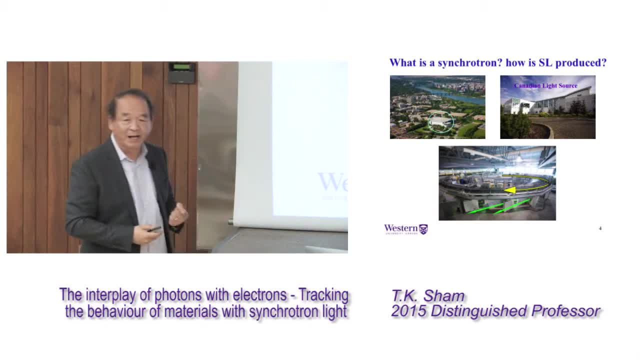 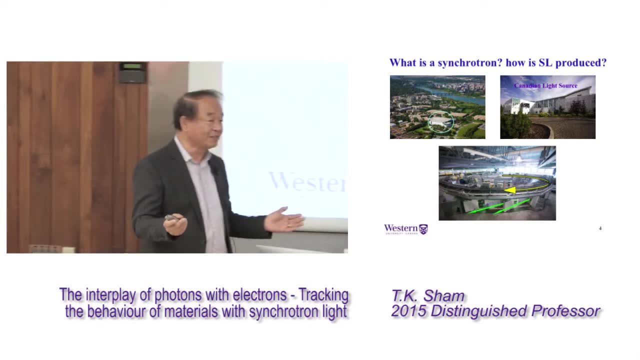 And this is the single trough line right. It's a really bright beam of light and it's highly collimated, all right. And also within this light beam you have all the photons, just like that. So this is the cardinal right. 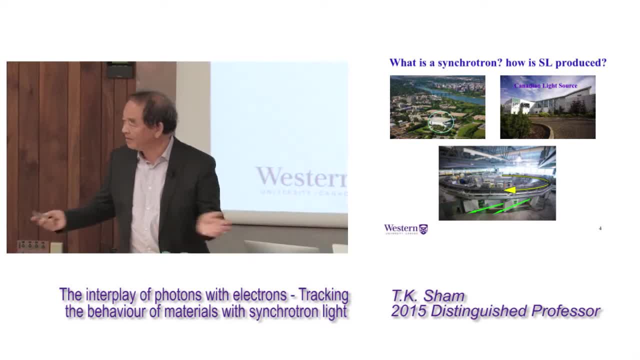 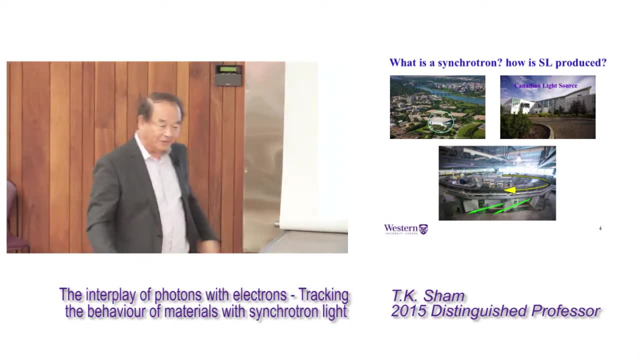 You have infrared, you have X-ray, you have UV, you have visible, you have everything. All are within this five beam of light. Okay, so another way of looking at light, or signature light, is to go to what we call. 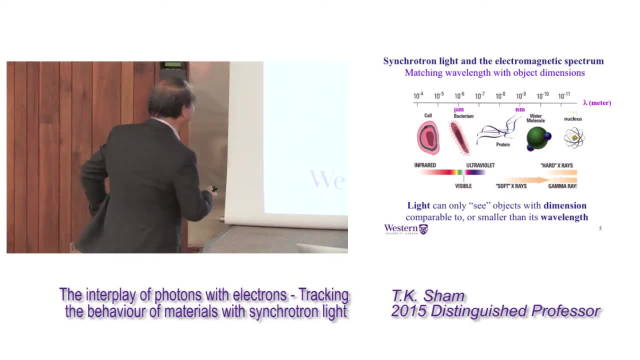 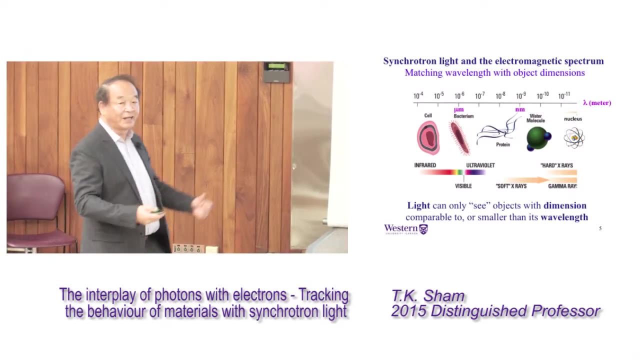 the electromagnetic spectrum, right, Okay, and here, historically, we like to give names to light with different names. For example, we have infrared, we have visible, we have ultraviolet, UV and X-ray and gamma ray, and so on. okay, 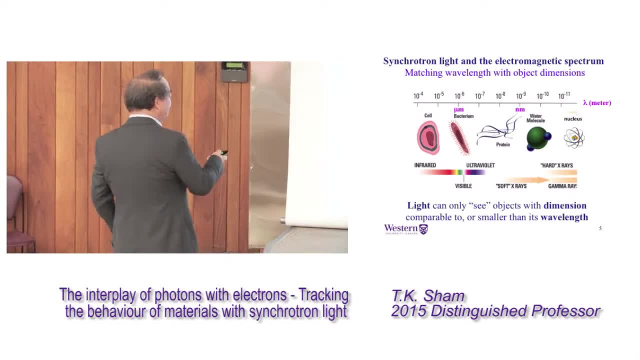 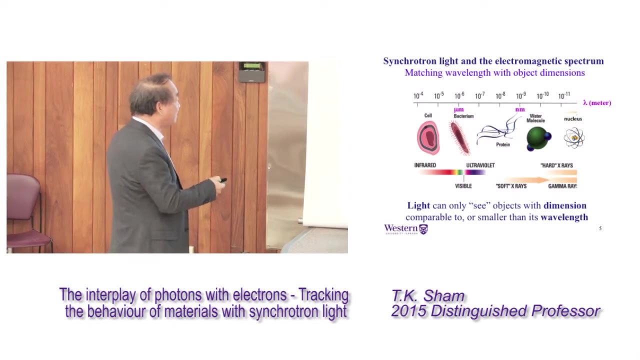 So we give them names. In fact, we can also match the wavelength of all different light with the size of object. For example, the size of material is comparable to the wavelength of visible right, Say, a water molecule. its dimension is comparable. 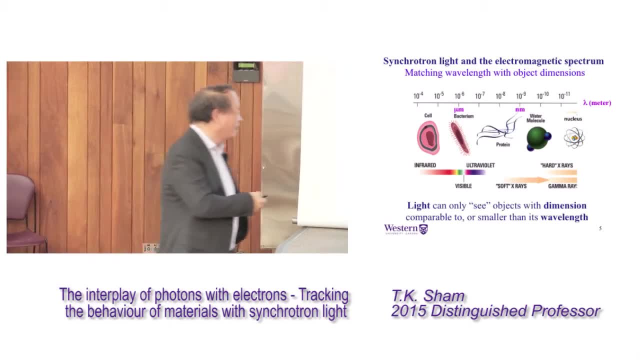 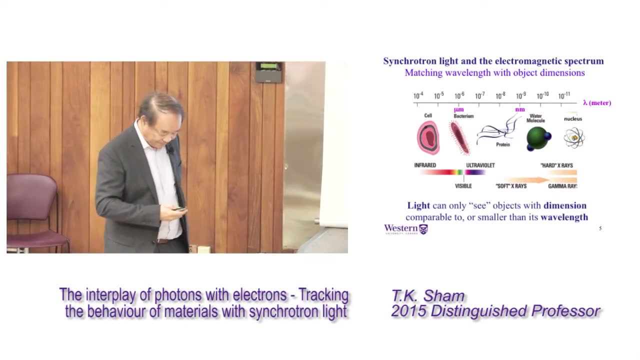 to the wavelength of X-rays And the nucleus its size is comparable to the wave of gamma rays. So this is one of the very interesting property of nature. I'm saying all of this because light can see objects. You usually like to see objects, right. 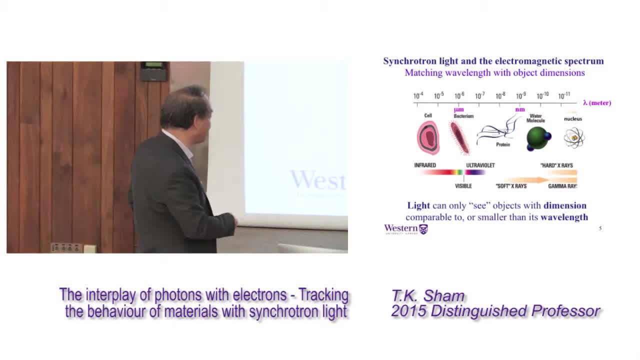 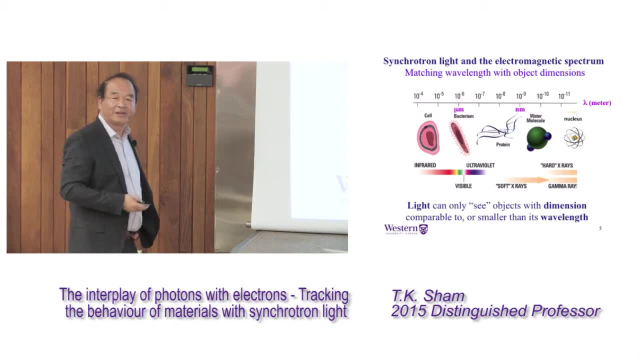 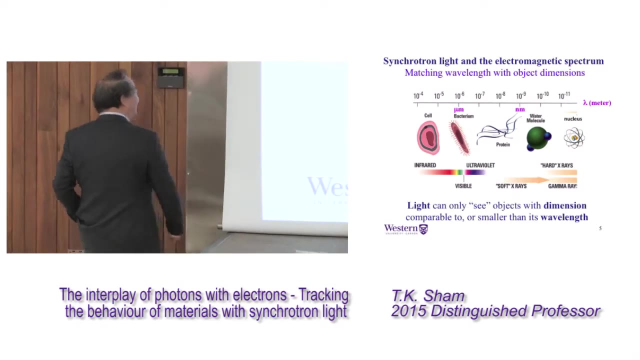 And only when the dimension of the object is comparable or smaller than its wavelength. Right? if the object is too small, then you cannot see it. if your wavelength is too large, okay. So let me illustrate this by doing a measurement of a daily object. 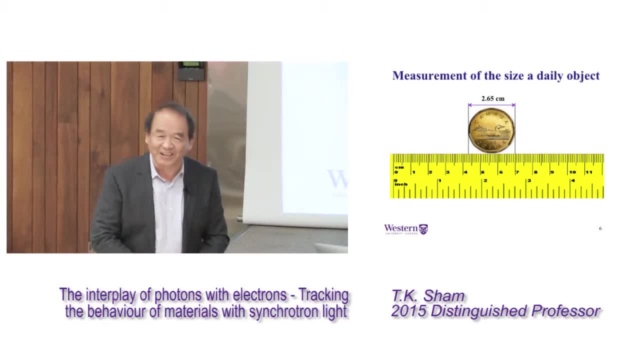 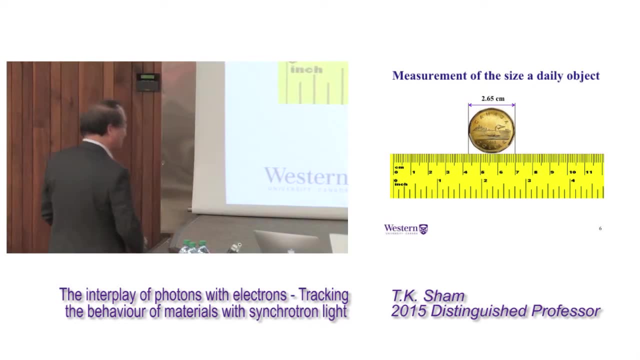 What is the most popular daily object? Possibly a loonie right. So let's look at a loonie, and what size is it? So let's bring in a pupil, a cerula. all right, Pupil, cerula, and then you can eyeball it. 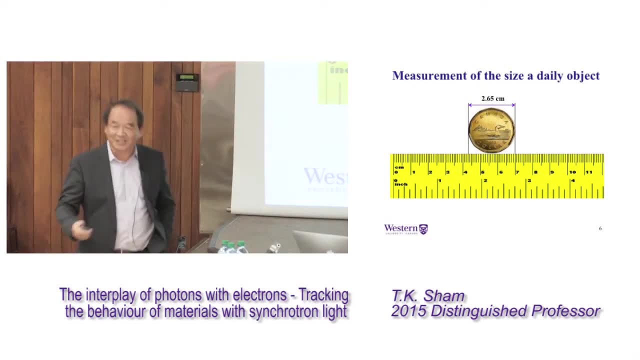 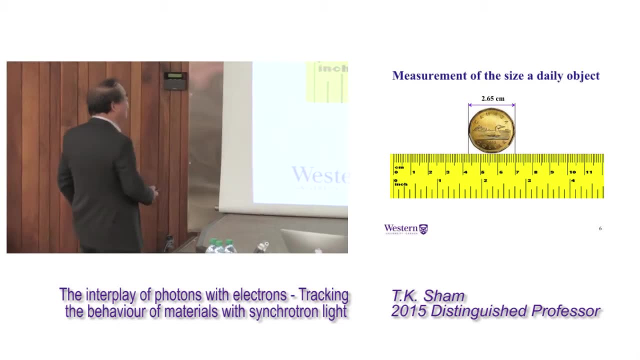 looking at the marks, looking at the division, and then you say, ha-ha, this is 2.65 centimeter in diameter. So that's the. then you can do measurements with a ruler of daily object. But how about hair, human hair, which is not finer? 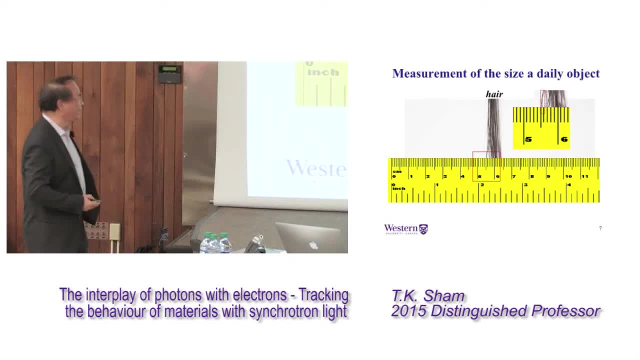 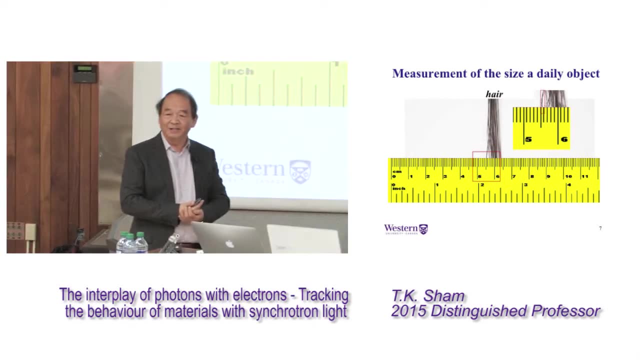 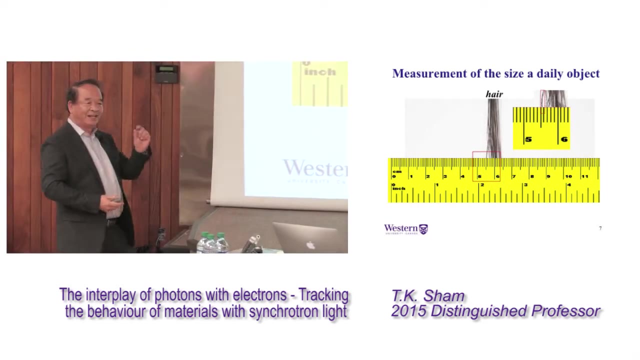 If you bring in the same ruler, then you realize that the interval between the division is just too large. so you cannot use a pupil cerula to measure the dimension of a hair, the size of the hair. So what do you do? You have to find a ruler that has marks. all right, 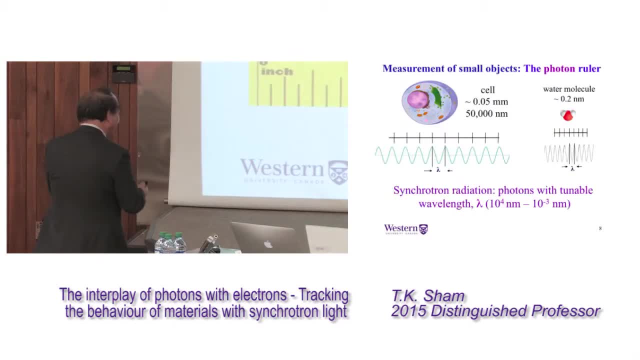 where it has smaller intervals, You have to find a mark. So that's where the so-called photon ruler comes in. For example, if you want to measure the size of a biological cell, which is typically of the order, say, 0.05 millimeter or even smaller, 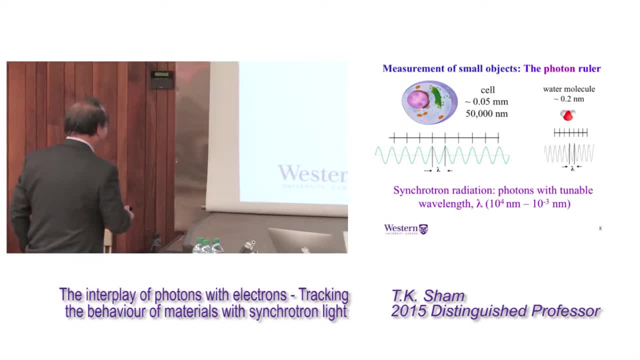 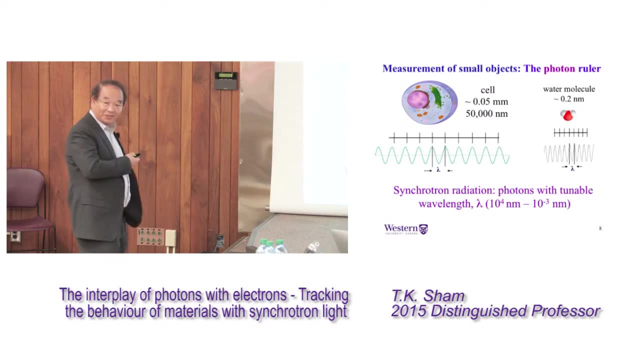 arctic light water molecule. all right, Now, to do that, you definitely need a ruler with marks, and you have to find a ruler that has a smaller interval than the object itself, so you can measure. all right, So this is what the photon ruler comes in. 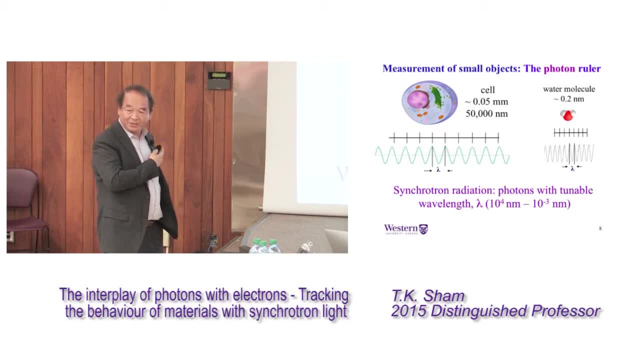 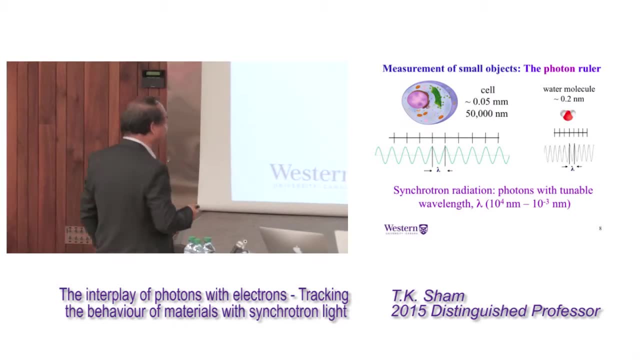 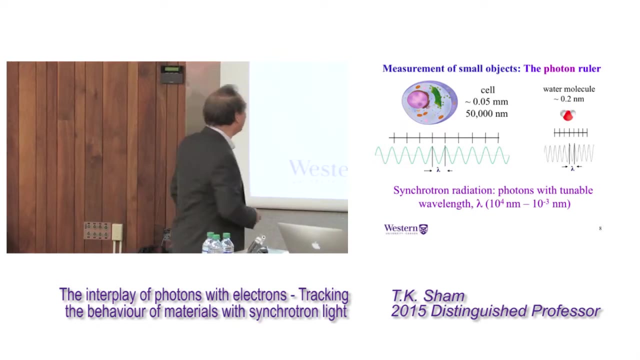 and the wavelength is the interval of the markers, They'll allow you to do proper measurement. So if you want to go to measure a water molecule then, which is a lot smaller, then you need light with much shorter wavelength. okay, So that's how you do measurements. 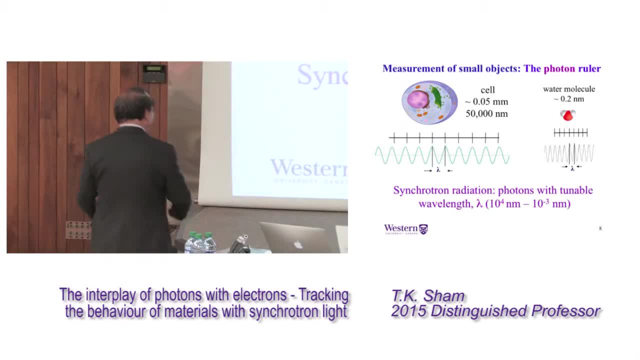 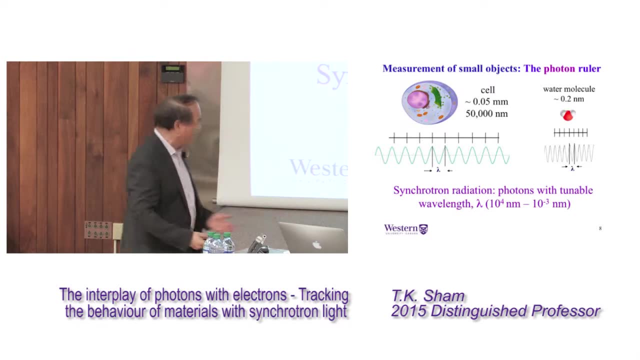 with light. so that's why I call it the photon ruler, Now synchrotron. why do we use your synchrotron? Because synchrotron provides all these rulers right. You can have whatever size you want. So the next thing is: how do we use light? 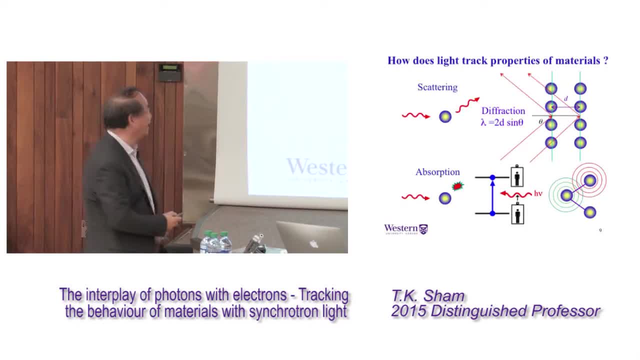 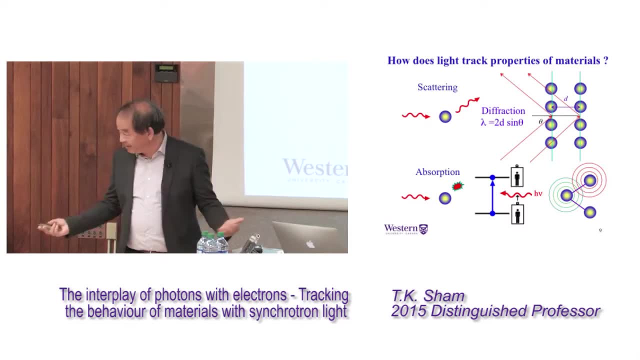 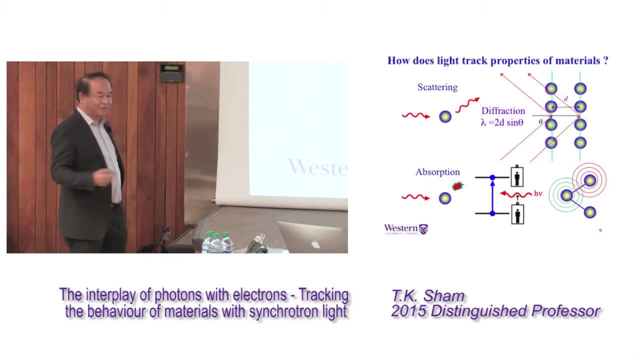 to investigate the property of a material. okay, And light interacts with material in two ways. In fact, they're taking place at the same time, So these two phenomena are occurring at the same time. So first is scattering, Let's say a photon comes in, interact with an atom. 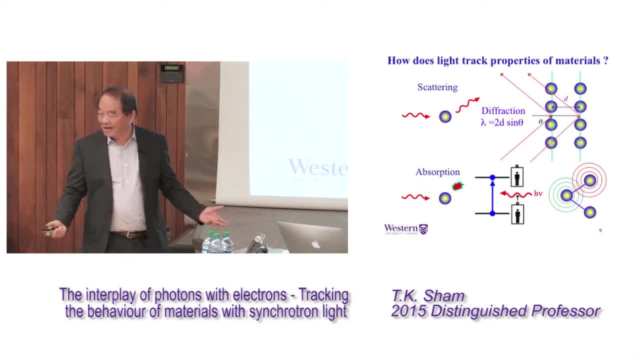 So this photon can get bonds in all directions. How it gets bond really depends on the wavelength and the property of the atom, right, Whether it has a lot of electron or doesn't have a lot of electrons. And when atoms come together they can form a crystal. 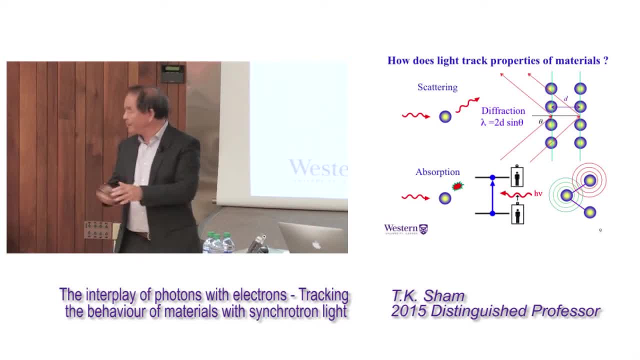 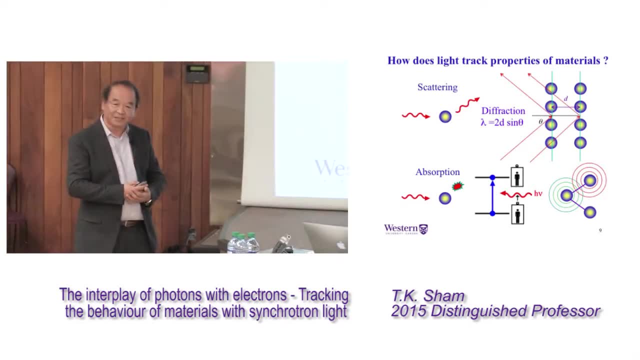 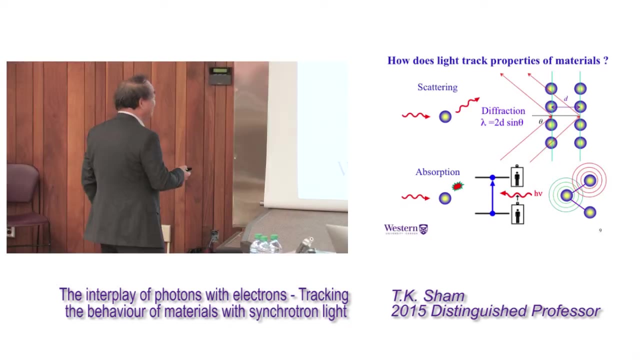 So the atom can line up in the crystal to give you lattice planes, And this lattice plane can diffract and scatter the light coherently, And the term for that is diffraction. So if the light we use is correct to certify the so-called diffraction condition, 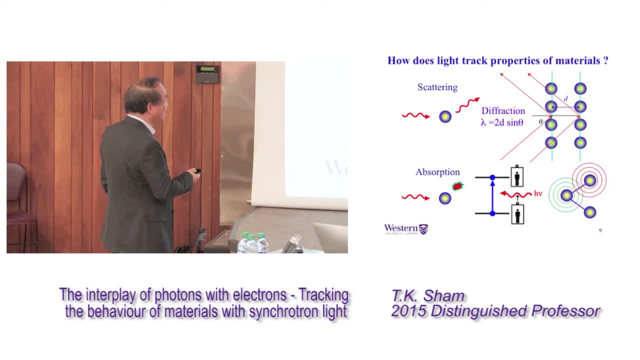 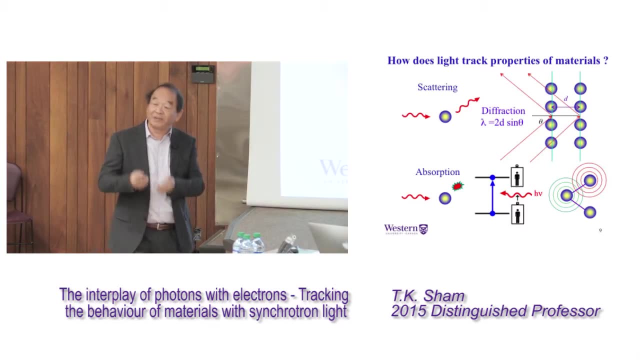 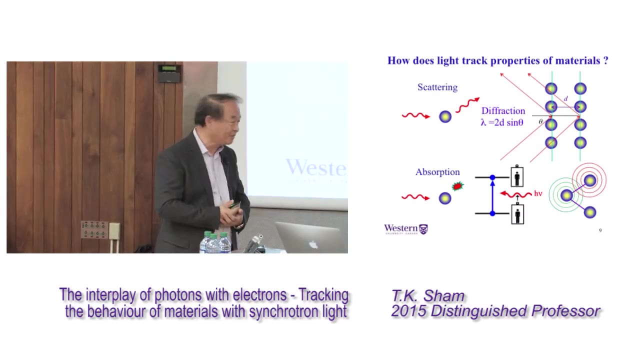 where the lambda is the wavelength, the d is the lattice spacing and the angle of fader is the angle of incidence. If that happens then we can get diffraction spot of the light And from the diffraction pattern we'll be able to determine the structure of the material. 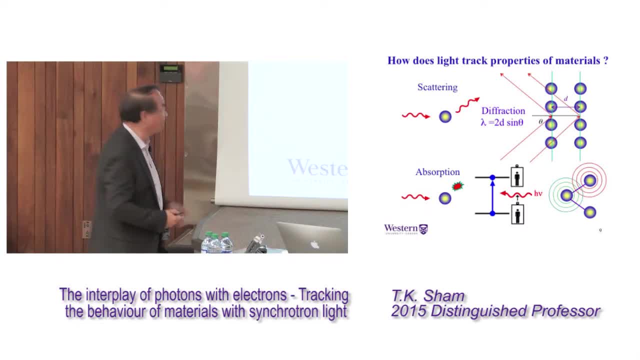 So what element you have in there, how far are they apart, and so on. So another phenomena is called absorption. Photon comes in right And just like a car crash, So you cannot salvage it, So all the energy is gone. 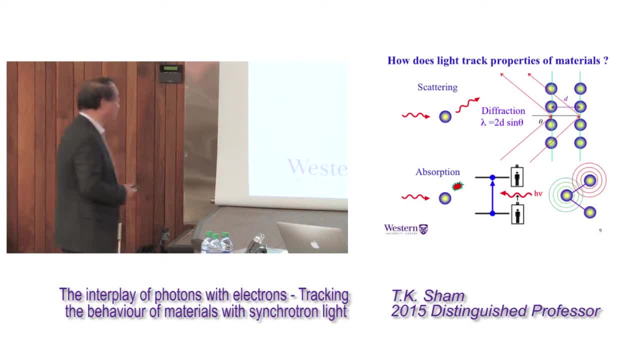 So the energy of the light comes in, it's all absorbed And the energy goes into the system right In the excited state. So this is just like most of the time, all the energy the photon has is given off to the light. 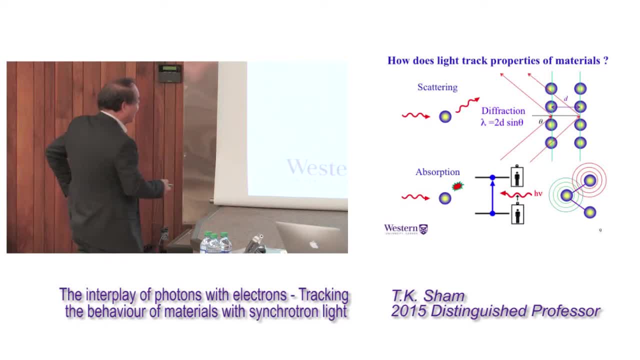 So the light goes into the system. It would take an electron from the grind state, so to speak, to the excited state, Just like electron taking an elevator right. So it gives some energy, it goes from a grind state to the excited state. 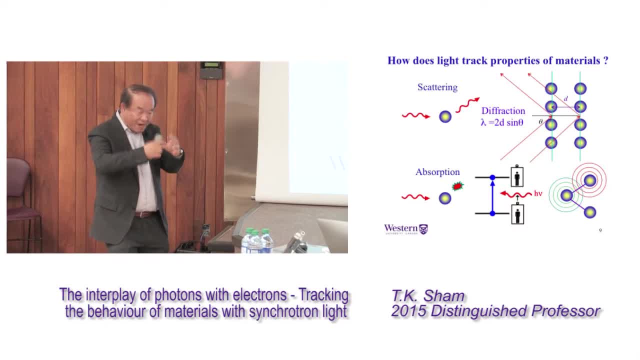 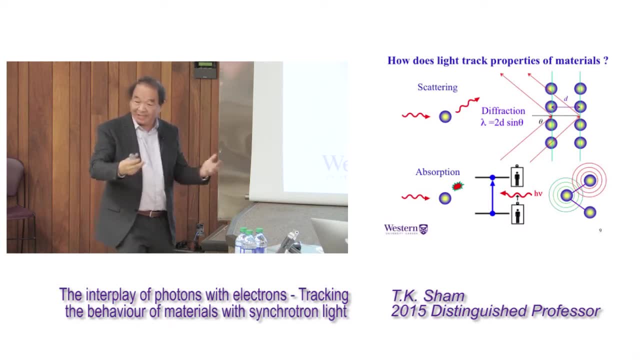 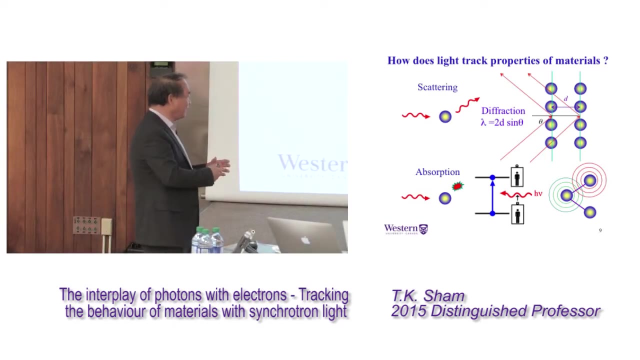 Now in a molecule the same thing happens. An excited electron actually can probably get away from the atom, right So? and then it gets bounced around by the laboring atom, just like a radar, right? So the information gets bounced back to the laboring atom and the result of that? 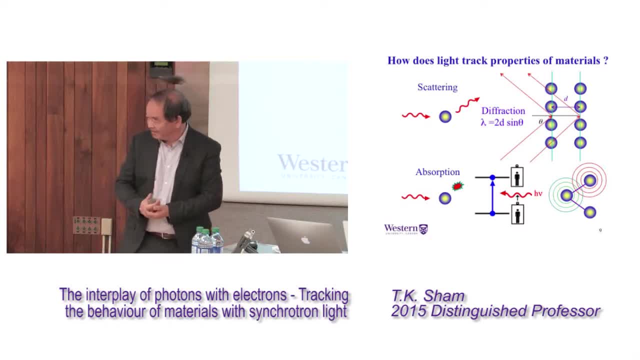 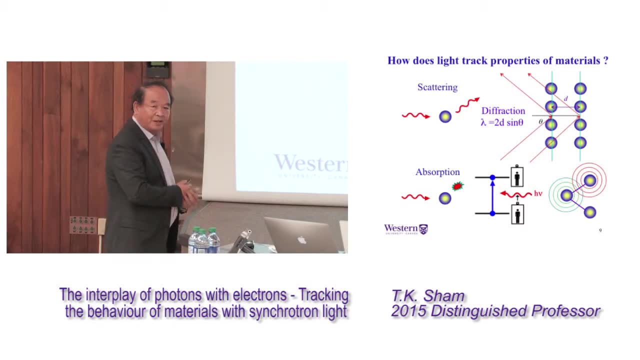 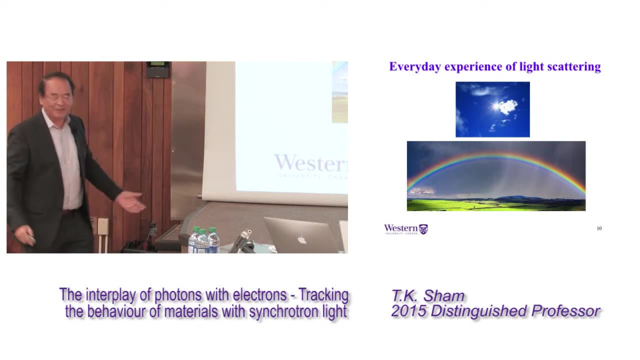 gives you all the information about the laborehood. This is the atomic laborehood, okay, So therefore, by doing absorption and scattering, you can get a lot of information about the structure on the atomic level. Now here's some of the everyday experience. 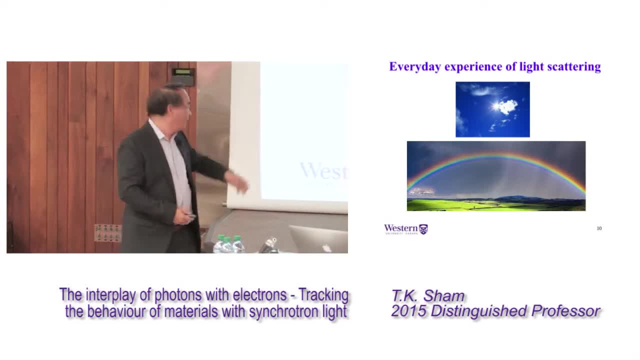 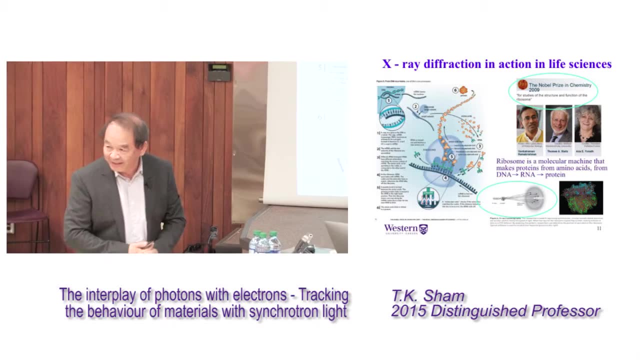 of light scattering and you all know that We have blue sky and we have rainbow after the rain. It's improved because of light scattering, But in the laboratory things can get more complicated, But it's still light scattering, but you can use it to do something. 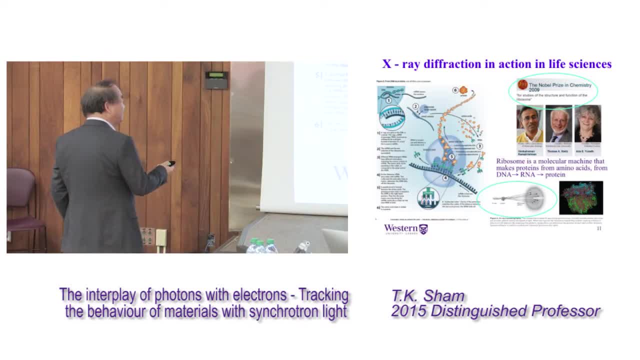 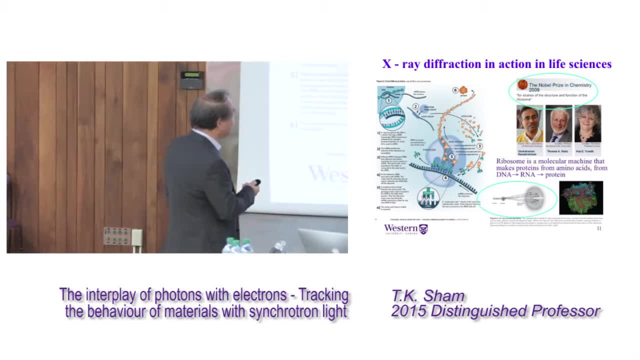 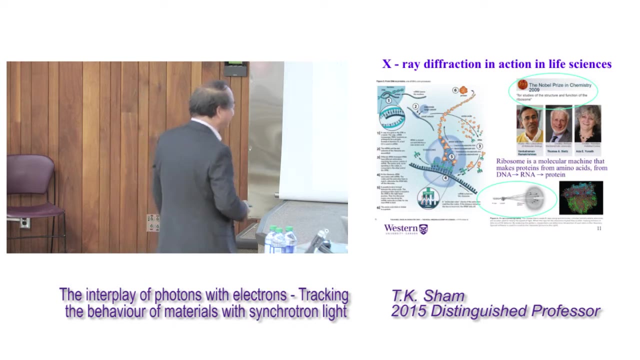 So here I'm going to use the Nobel Prize in Chemistry in 2009 as an example. Now these folks won the Nobel Prize for their study of the structure and function of ribosomes. Now, ribosomes is a very interesting entity. It's the molecular machine that makes proteins right. 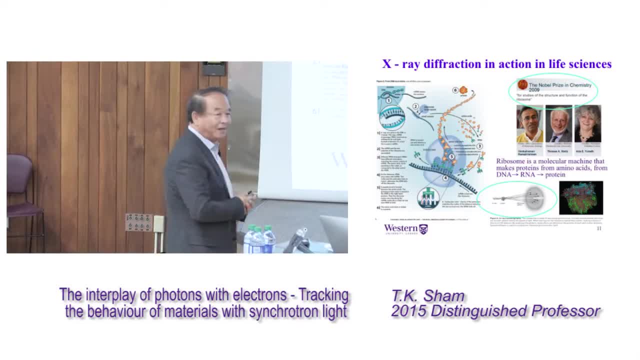 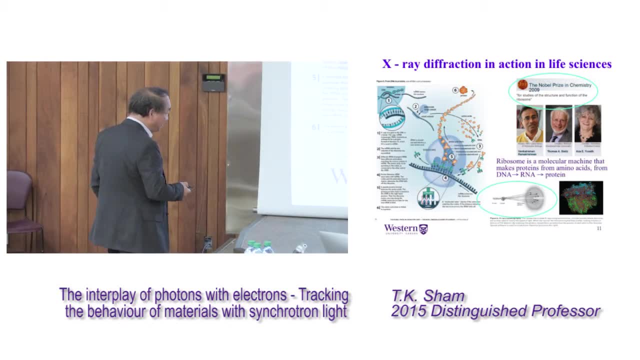 So to understand how it functions, you really have to know the structure. And the structure entry was determined using X-ray from the singletron right. You cannot do it in the laboratory, You really have to use the singletron line. So, and these folks figured that out. 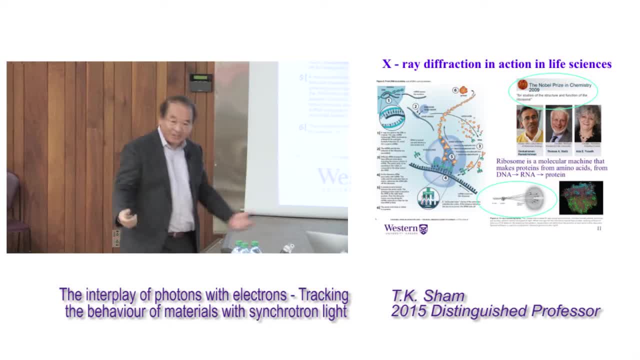 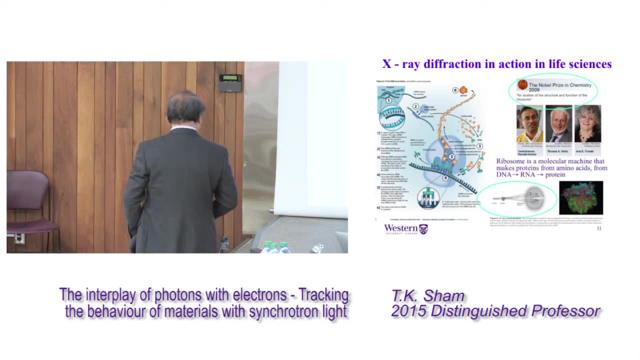 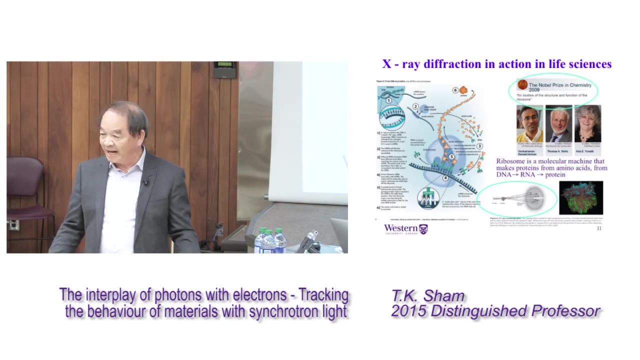 and they determined a very complex structure, but still a simple phenomenon: light scattering. okay, All right. so here I want to give you another example of X-ray absorption. This is one of the most interesting X-ray image of all time. This is one of the very first X-ray radiograph. 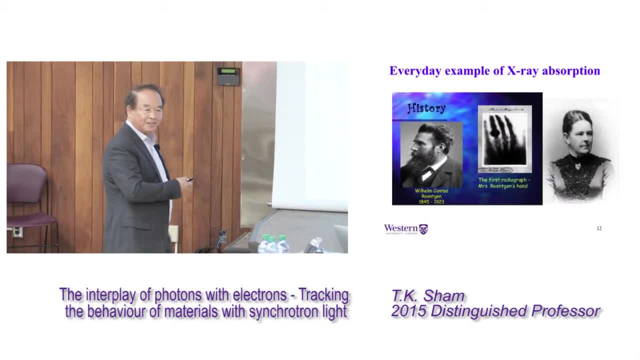 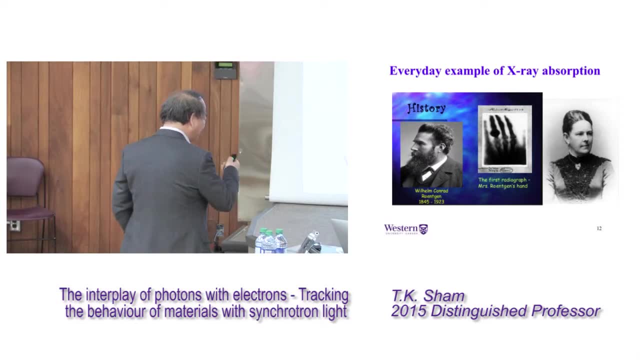 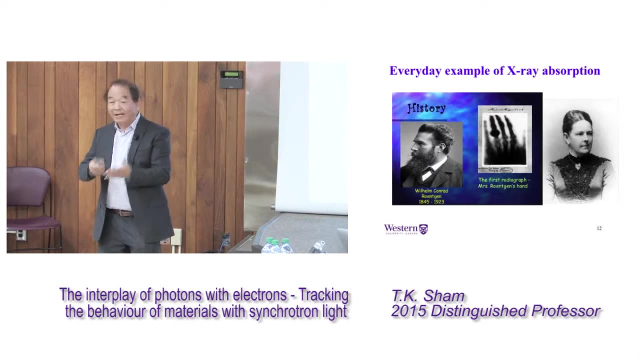 of the hand of Mrs Regens right, The wife of the German physicist who discovered X-rays. Now, the reason you actually can see an image is because you have skin, you have flesh, you have bone and then you have the retina. 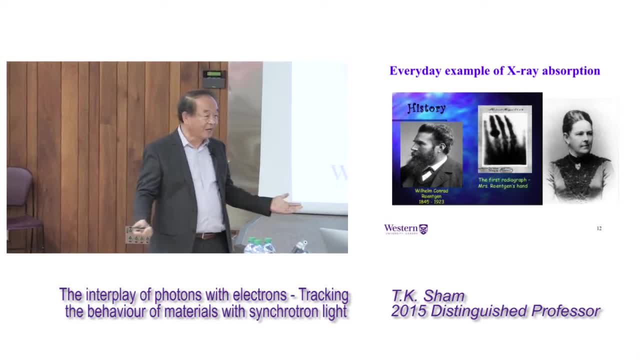 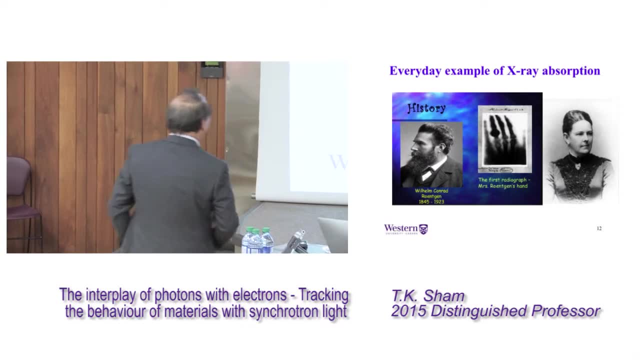 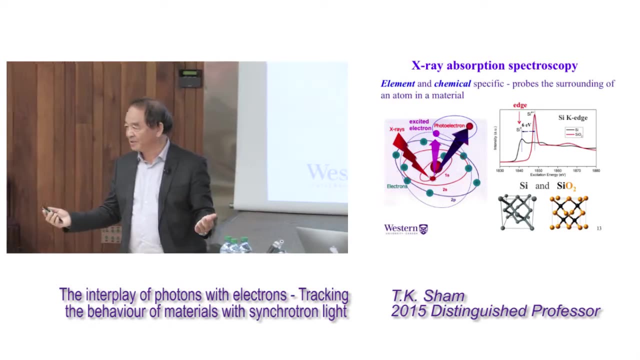 They all absorb X-ray different. It's the result of that: You get contrast, you get image and you know what's going on. okay Now, so this really comes down to what I've been doing right. So I've been using X-ray absorption as a tool. 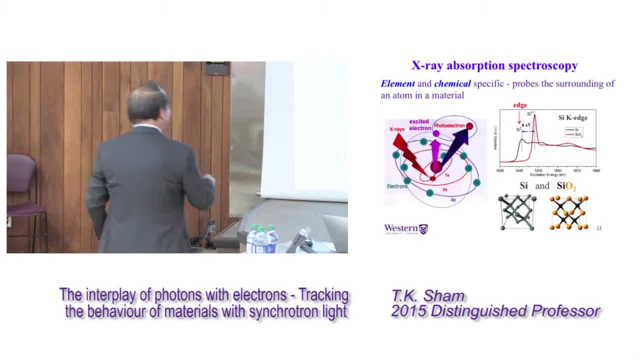 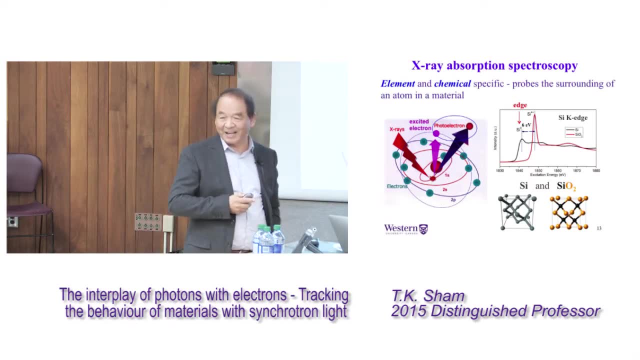 to look at all kinds of stuff. okay, Now, X-ray absorption, spectroscopy, is arguably the most powerful tool of all time. okay, And then I try to convince you that. okay, I'm pretty sure this is the case because it's element. 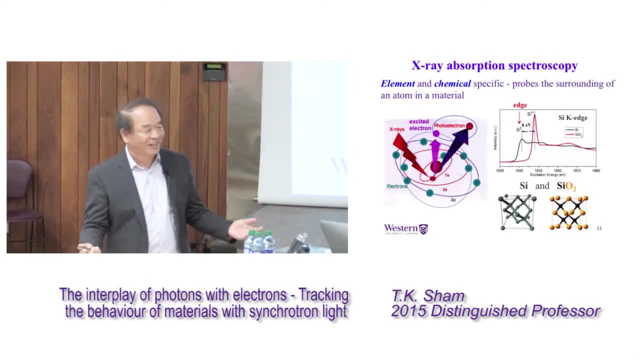 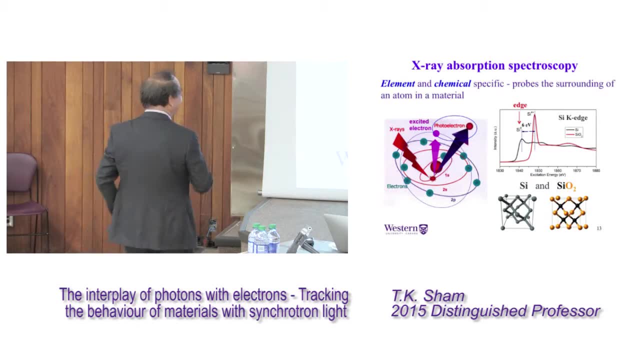 and chemical-specific. Well, everything had to do with element, and you and I have. we are made out of elements, right? So if you look at element, then you know everything In principle. in principle, okay. So you can probe the surrounding of a atom. 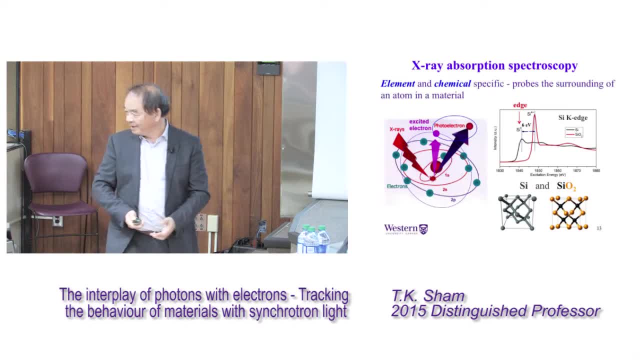 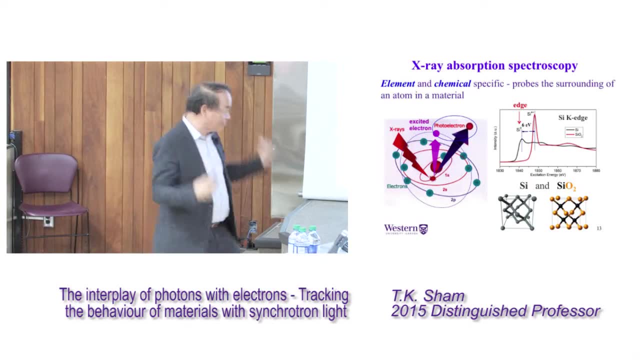 in the material or in any different environment. So this is how it works. okay, When X-ray comes in, it's JUDY, Yeah, sufficient energy. then you can excite a core electron, such as a 1s electron in any atom. 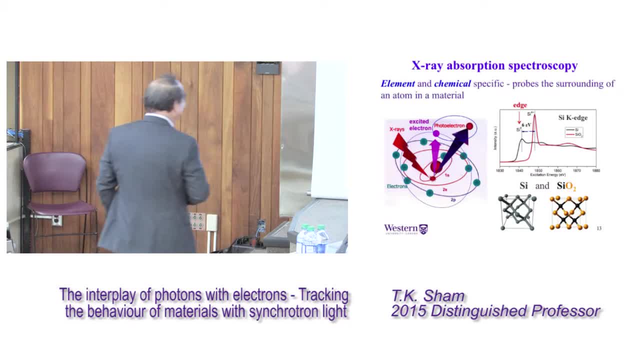 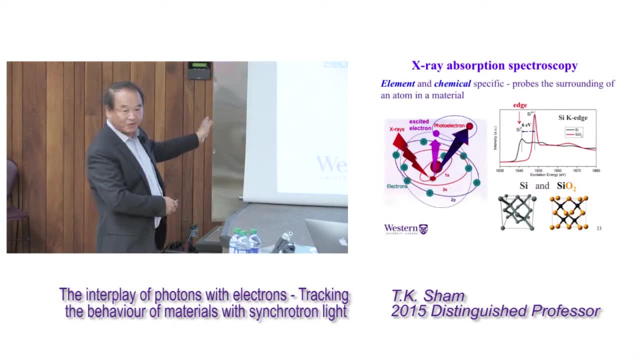 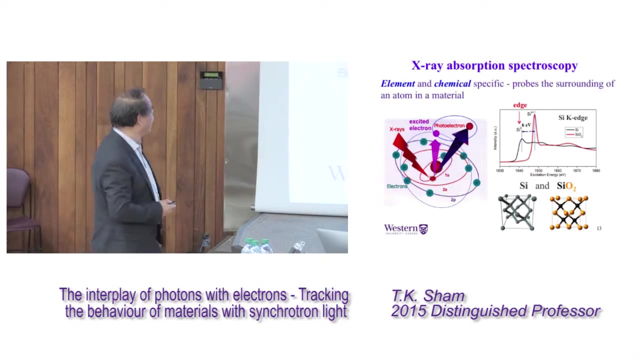 to the purest unoccupied electronic state, like a unoccupied atomic orbital. Okay, so now if you increase, so this is the threshold right, This is where everything starts. So then if the X-ray energy increases, then you can take the electron into the continuum. 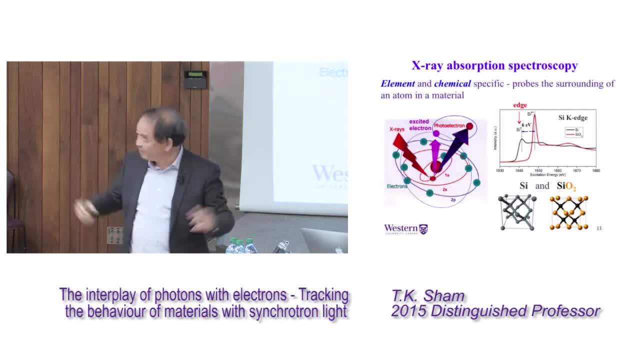 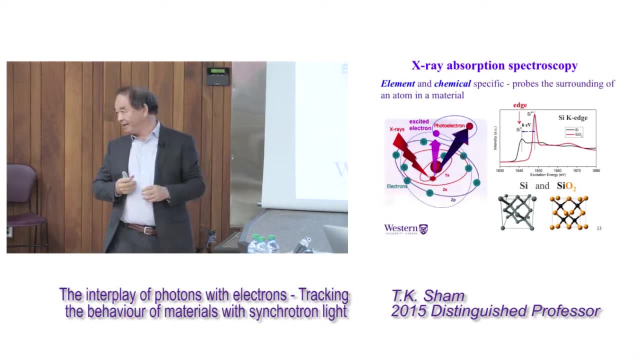 It becomes an excite electron which can travel away from the absorbing atom. Okay, when it does that, it gets bounced around by the surrounding atoms and brings back the information through bed scattering and because of the interference of the outgoing and bed-scattered. 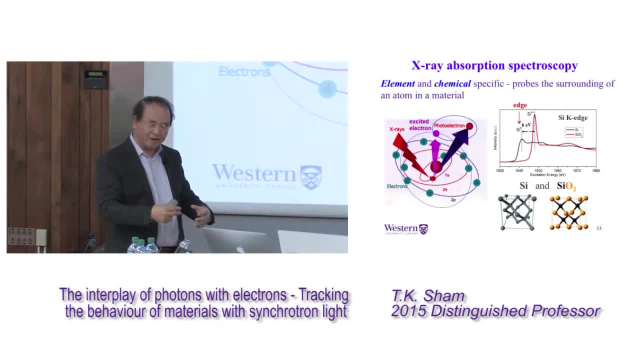 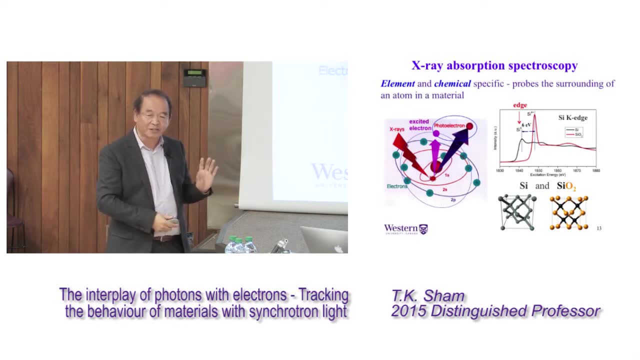 electrons. all this information got wrapped up, or accumulated, into something we call X-ray absorption spectrum. So, in principle, X-ray absorption spectrum contains all the information you want about the neighborhood of the atom that absorbs the X-ray. So let me show you an example. 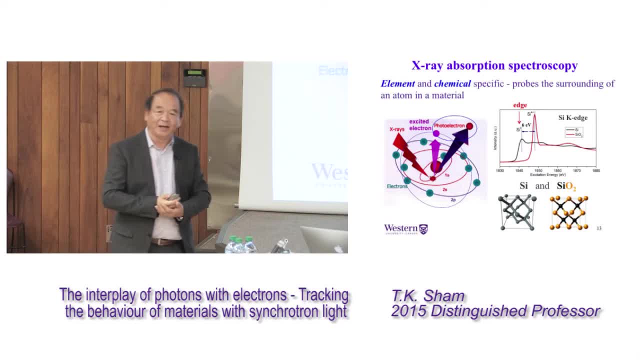 Now this is so-called X-ray absorption spectrum at the edge of silicon. Okay, at the edge of silicon. Here I show you two spectrums: X-ray absorption spectrum of silicon and silicon oxide. They basically have the same structure, but in 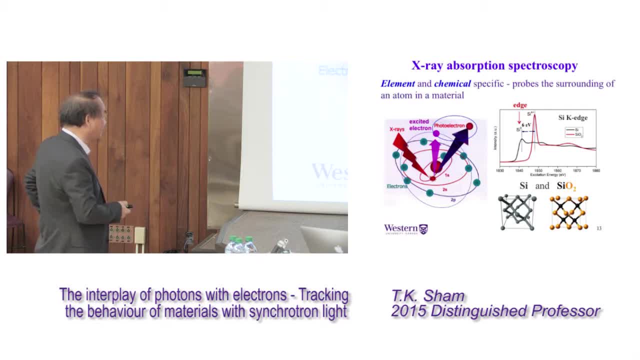 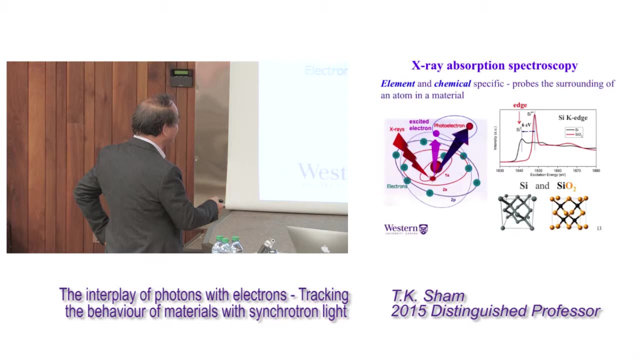 elementary silicon is surrounded by four silicon atoms. In silicon oxide, the silicon is surrounded by four oxygen atoms. Alright, so as you can see the absorbers spectrum, first of all you see a increase in the absorption coefficient when the energy that comes in 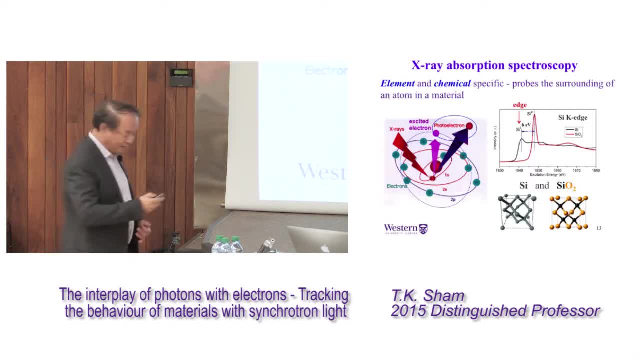 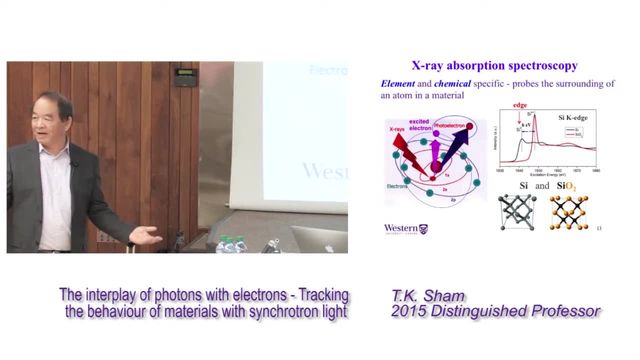 is sufficient to excite the electron. That's the threshold and thaty dragonylonide growth in that historical is called n teh, where absorption spectrometry always has to do with edges. right, Because edges tells you what element there is. 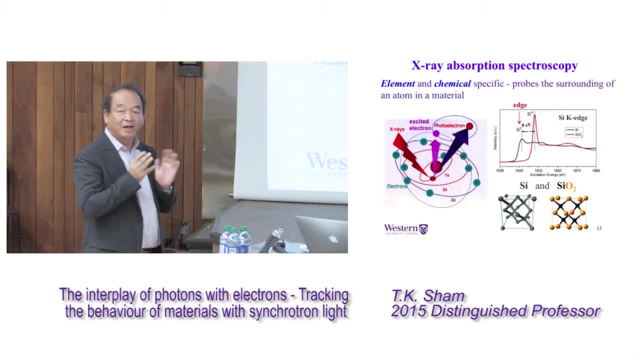 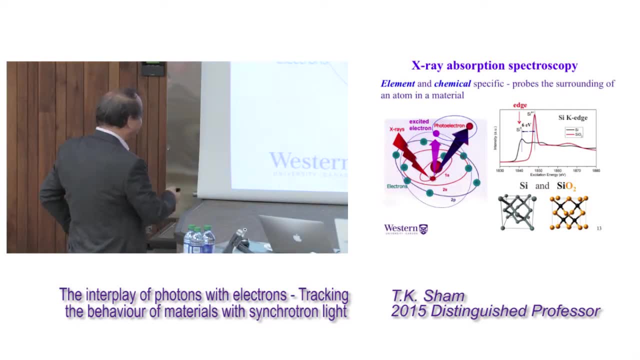 Because if you see some edge, a certain energy, you can only have that element, You cannot have anything else. OK, All right. And then beyond that, all this oscillation, beyond the threshold, are the information the electron brings back to their absorbing. 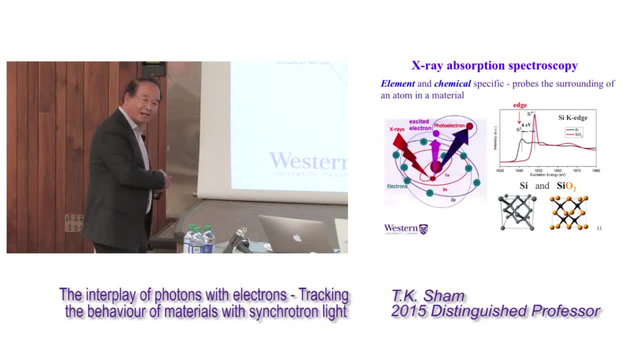 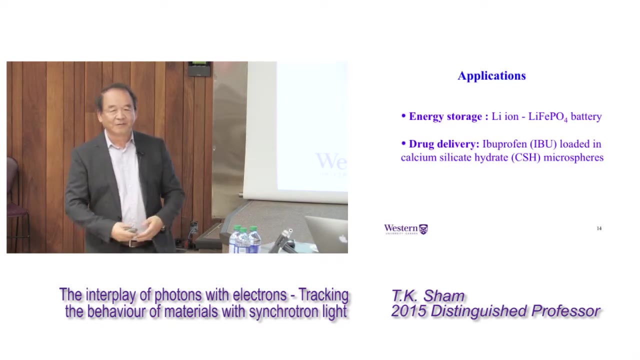 atom about the surrounding. So the trick is how to analyze it. If you know how to do that, then you know everything about the neighborhood of the atom. All right, So now I just want to illustrate some of the applications with two tiny examples, maybe all right. 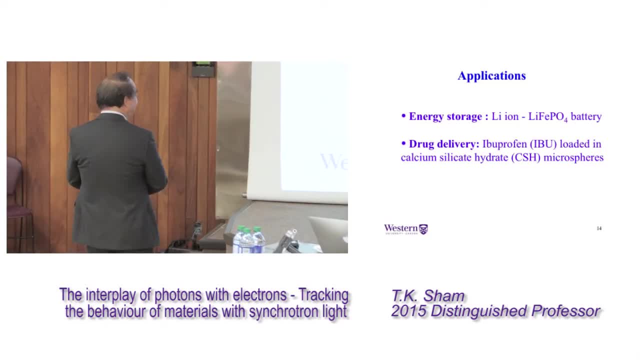 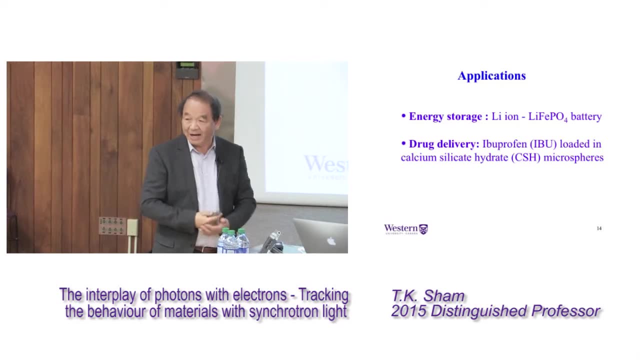 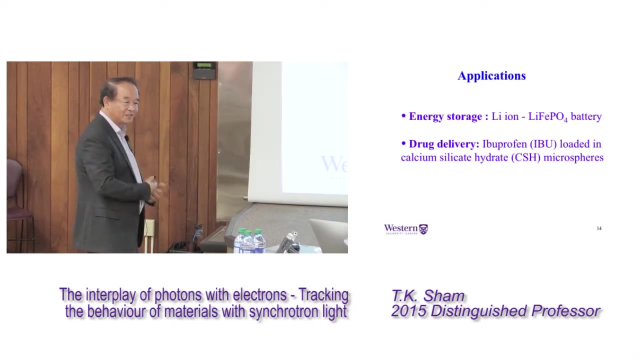 One has to do with energy storage in lithium ion- lithium ion- phosphate battery, which is one of the hottest subject of this time, all right, And the other has to do with drug delivery. How are we trying to know our own drug and deliver in certain system? 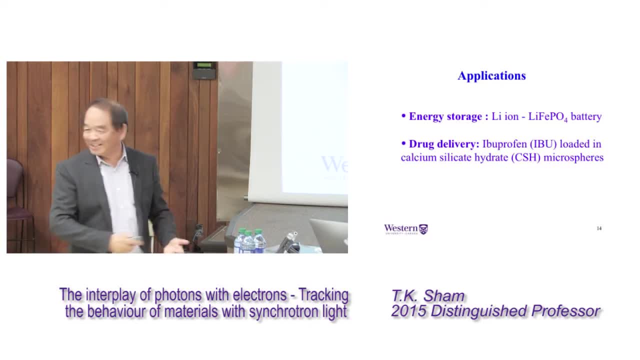 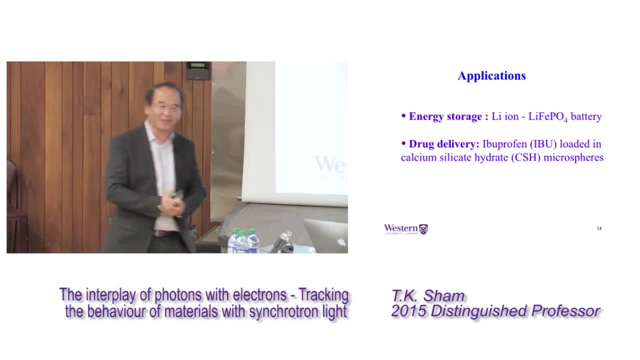 So how do we do it? Well, this has got to do with single drug, right? And I'll show you what this has got to do with single drug. OK, All right Now. most of you know high school chemistry, right? 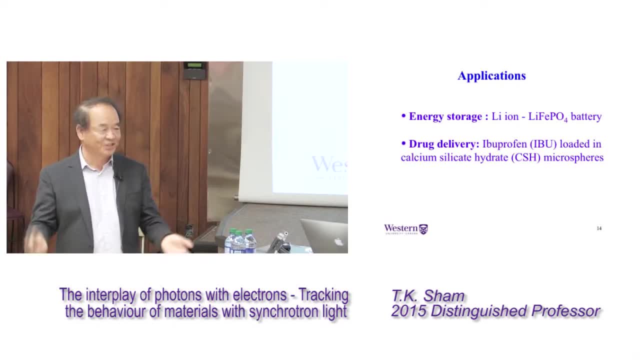 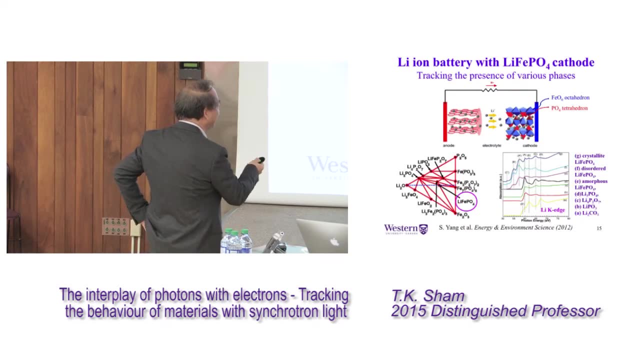 Electro battery operates electrodes. You charge and discharge, and so on. right Now, here, lithium ion phosphate is used as a capital. all right, All right, And this is the structure. So basically, you have alternating iron oxygen. 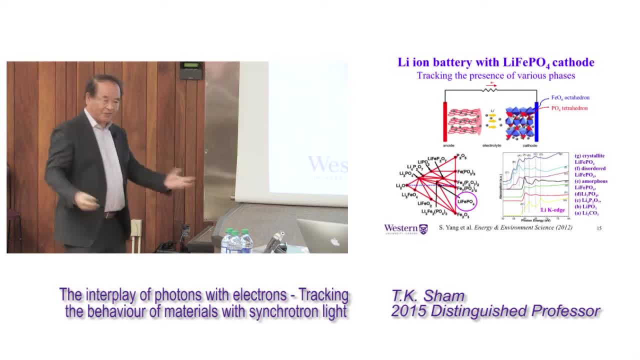 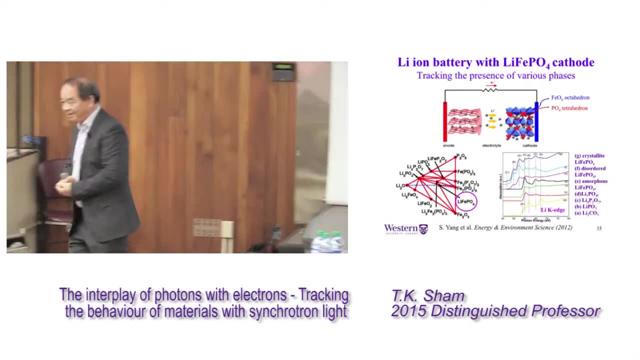 and phosphorus-oxygen polygons right, And then, in the space in between, you bring lithium in and out and that's it. That's your lithium ion battery, And that is it in principle. But we all know the devil is in the detail. all right, 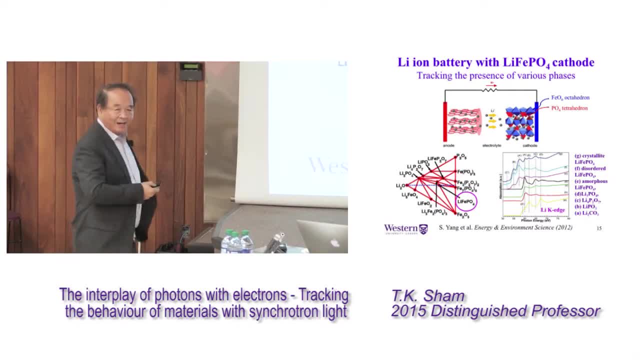 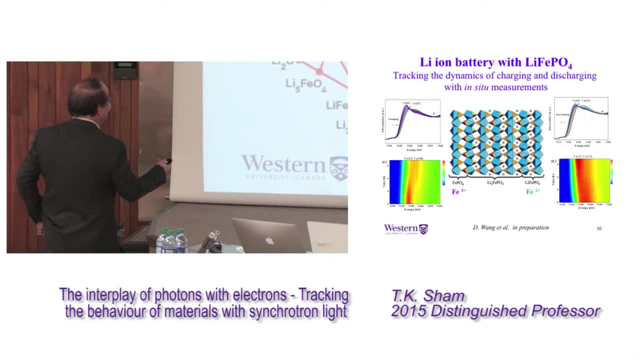 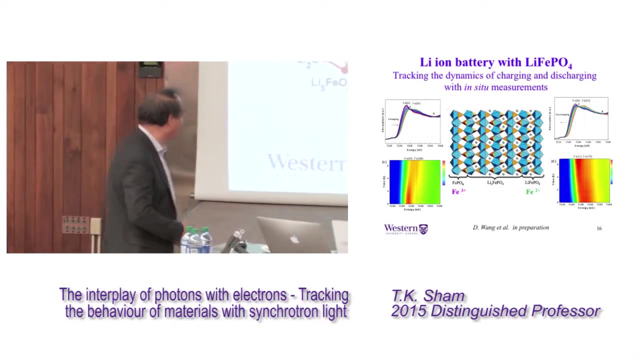 And here we go Now. when this happens- you know this battery operates from time to time- There are many, many various phase that are produced. Some people don't even know why they are there. OK, So this is where singletrons come in. 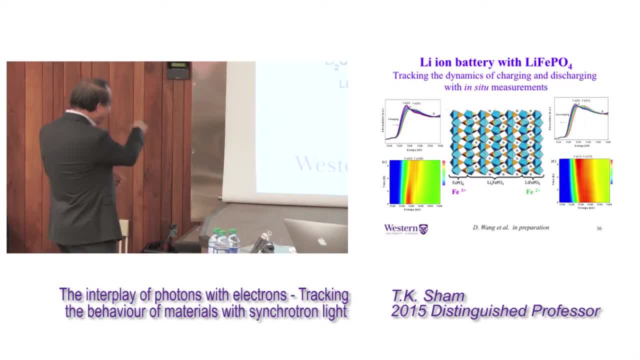 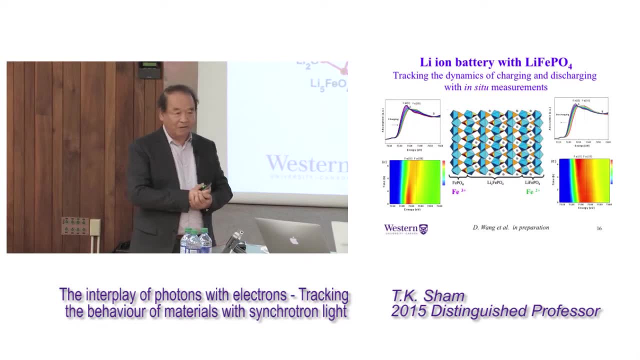 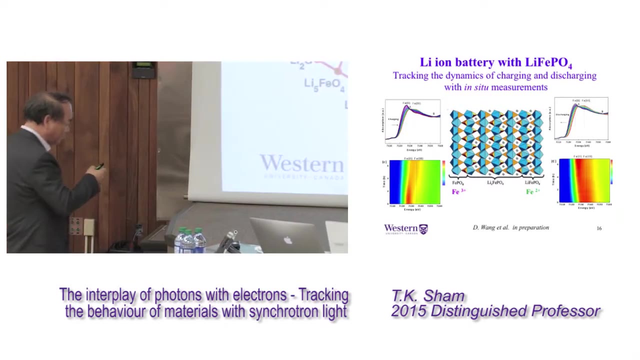 What singletrons can do is to give each and every one of these guys an identity, an X-ray identity. So then we know where they are and you can try to figure out how they are formed. OK, So By doing X-ray absorption spectrum here. 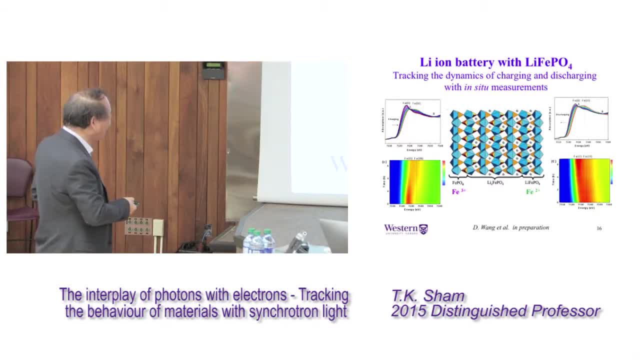 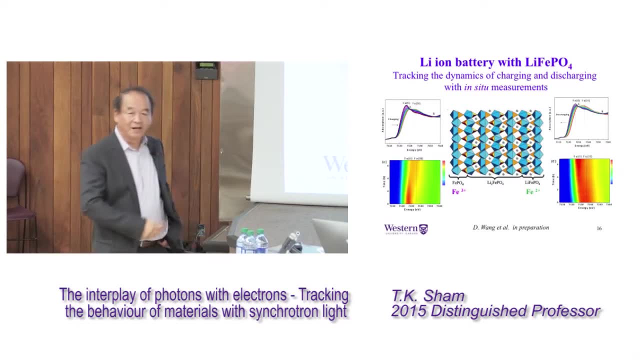 is the X-ray absorption spectra or fingerprints of lithium in all these different phases. We can do the same for iron, for phosphorus, and so on. OK, So that's one thing. You track the possible phases that can occur during the operation of the battery. 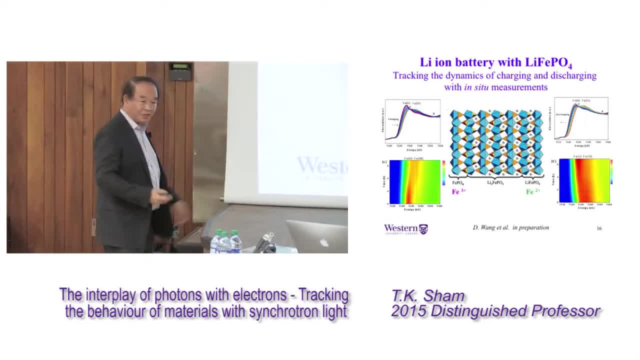 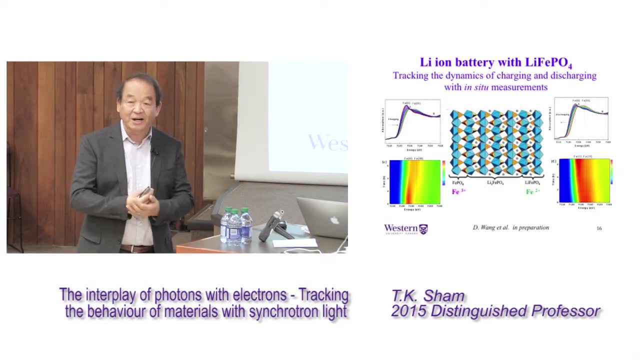 Now. another is that we can understand the dynamics of charging and discharging. Now, why are not, why we are not going to street cars, to electric cars yet? Because charging is really a problem, right, It takes hours, It takes hours. 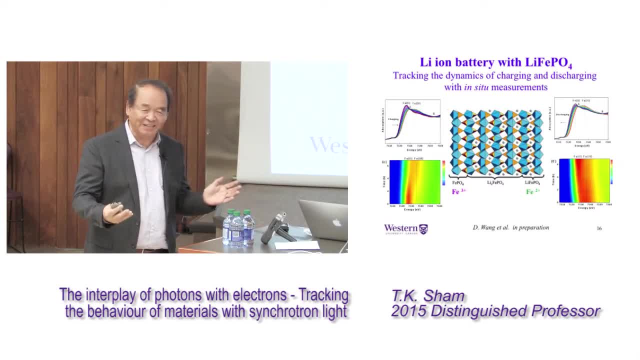 But if you go to the gas station, even if you want to fuel your tank right, probably five or 10 minutes. So understand the dynamics of charging and discharging is really, really important, And singletron can help you to do that by doing so-called in situ. 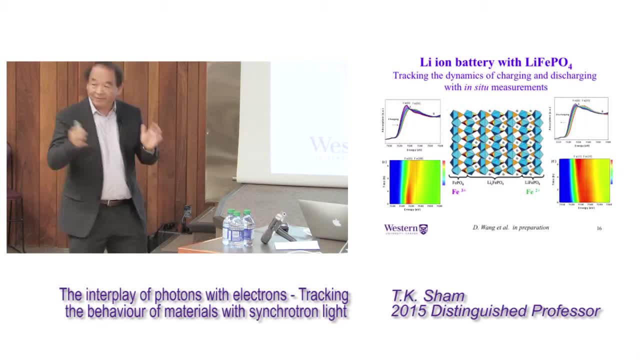 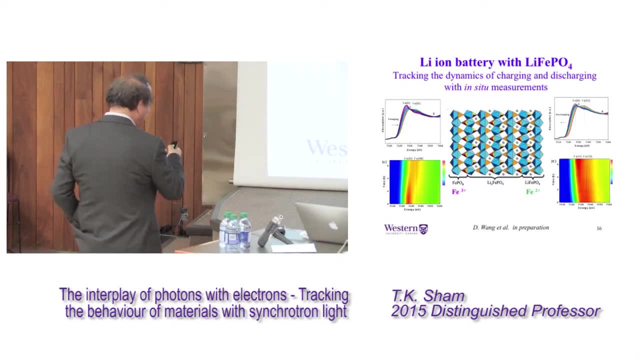 measurements. That means we are tracking the chemical state of elements in the battery while the battery is operating. OK, So now here is the scheme of the material at the cathode right. So on this side and that side are the system when it is fully charged or fully discharged. 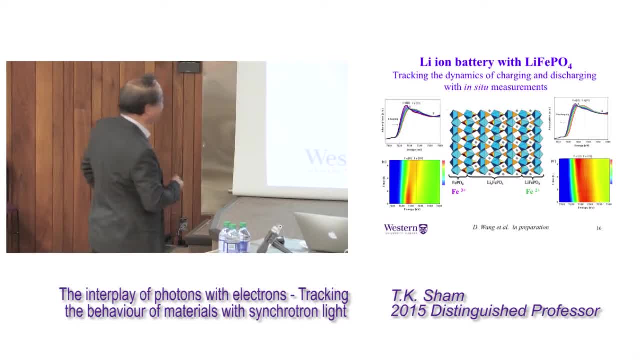 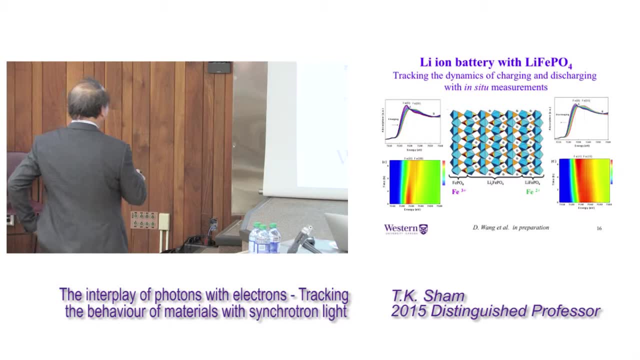 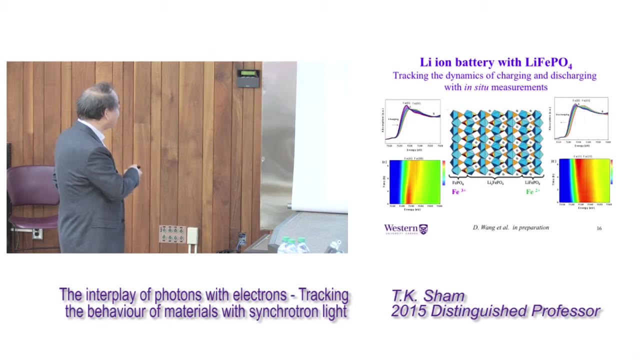 where here is somewhere in between. So by tracking the chemical state of an element of iron while the battery is operating, say when it's charging, and we can see the chemical state of iron in the material is changing When you're doing this measurement, as a function of time on the fly. 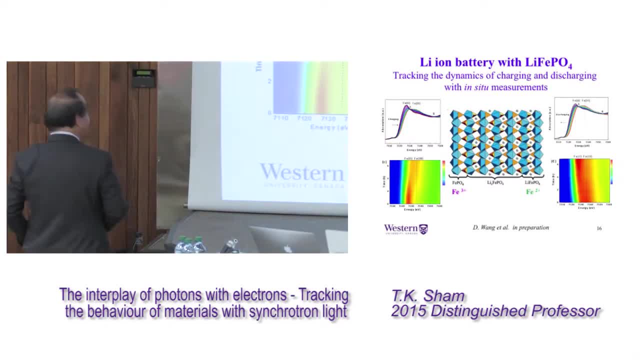 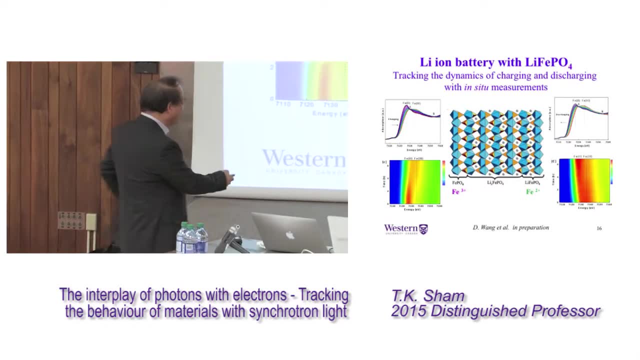 on the fly. that's in situ right, And we can also do the same thing when the system is discharging, That means when you put a node on it, And you can study the chemical change in a 2D map as a function of time. 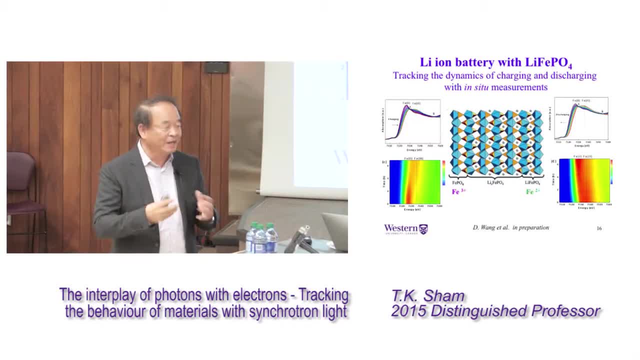 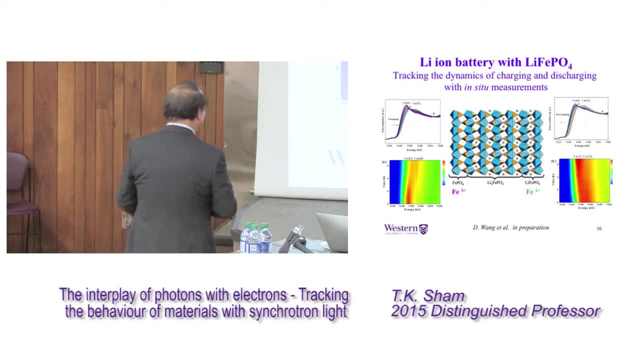 And by doing this kind of analysis you begin to be able to understand how the thing charges up. So this would affect the performance of the material. So the next example has to do with drug delivery in principle, right, in principle. So one of our approach is to try to load some of the drug. 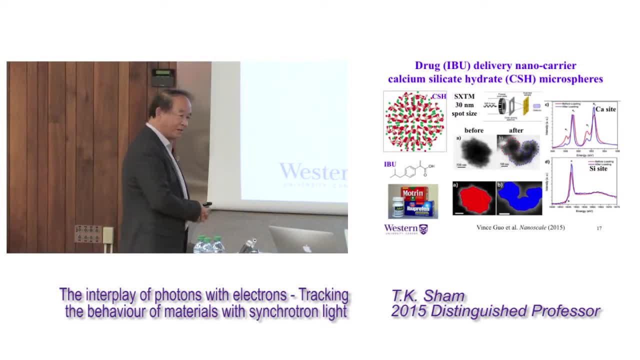 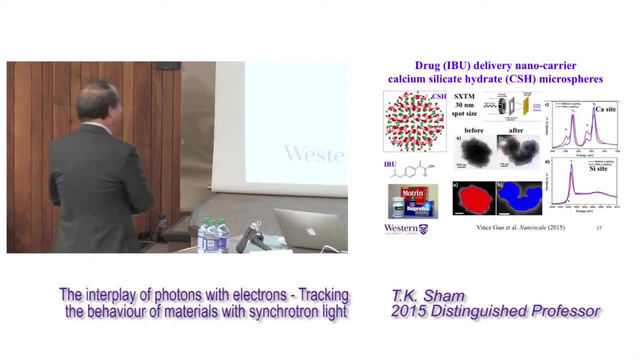 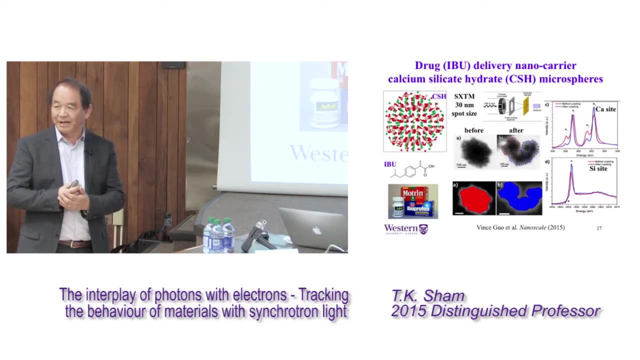 on some really cheap stuff. right? Calcium silicate hydrate microsphere- right, They are everywhere. right, It works. And the idea is the following: You start by making this material into microprocessor. This is a micro-sphere, okay. 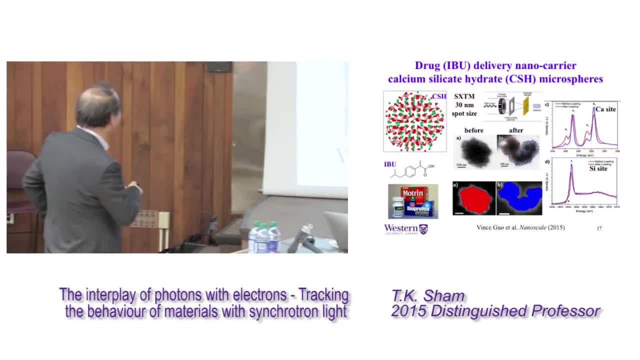 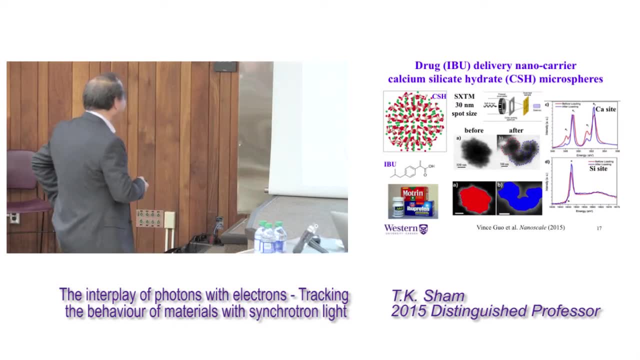 And it looks like this. It has a lot of porosity in that. And then we load this drug, the ibuprofen. Ibuprofen is an on-the-shelf drug that you can buy in the software's drug And it's available under various trade names. 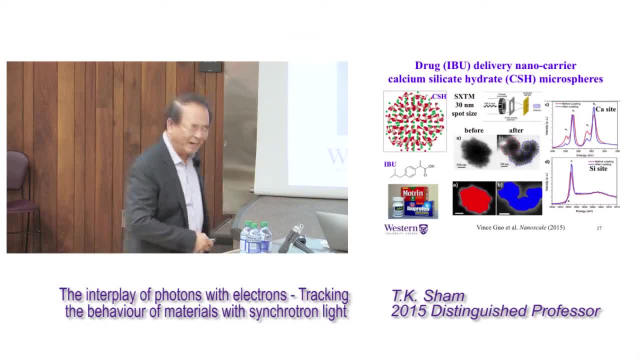 such as Motrin or Advil or things like that. okay, Now the tool we use. so what we are trying to understand is this, right. What we are trying to understand is how, in order for to do drug delivery, 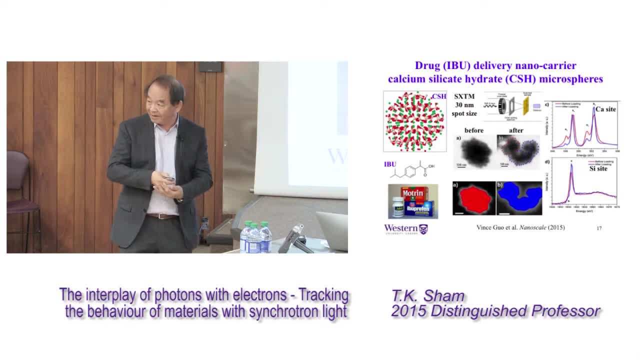 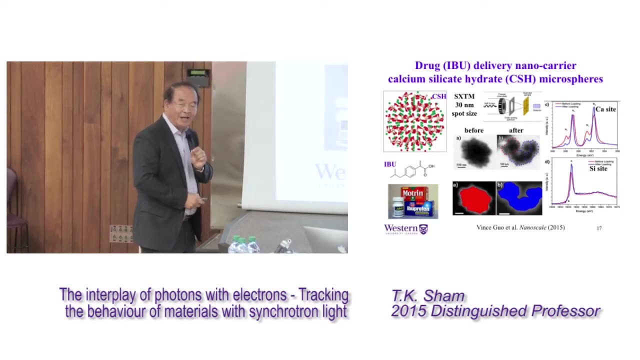 you have to know how the drug is loaded and interacts with the carrier. all right, So we do it with a technique called scanning, X-ray transmission microscopy. So we bring in a 30 nanometer beam which is very tiny. Now, a human hair is about 100,000 nanometer. 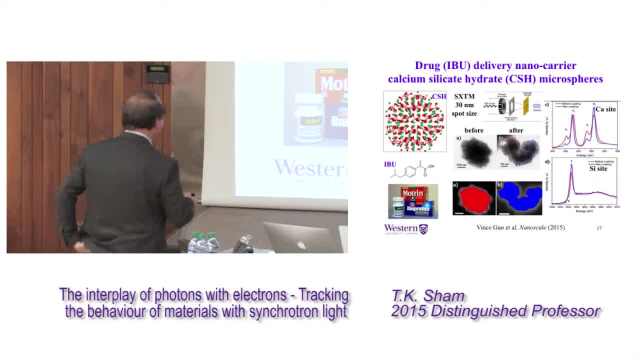 So this is 30 nanometer, Okay, so it's very, very tiny, And then we can look at one individual microsphere. We are not looking at the whole thing, We just look at one individual sphere, And then we can get the image before and after loading. 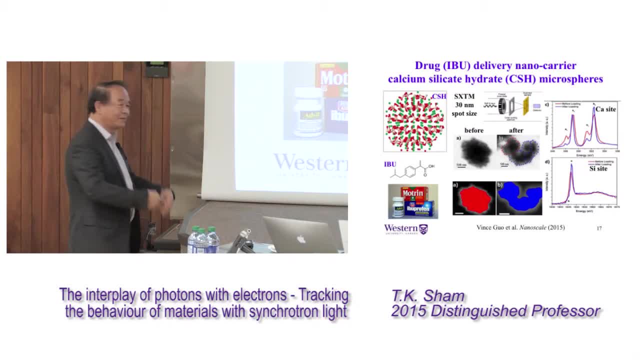 all right Now, of course, to do before and after loading. we have to use a similar batch. We cannot difficultly find exactly the same thing. fish it out, do the experiment and put it back in, Because this guy is only about 500, about one micron, right. 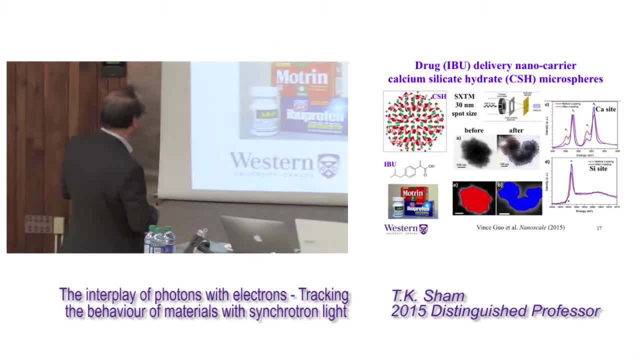 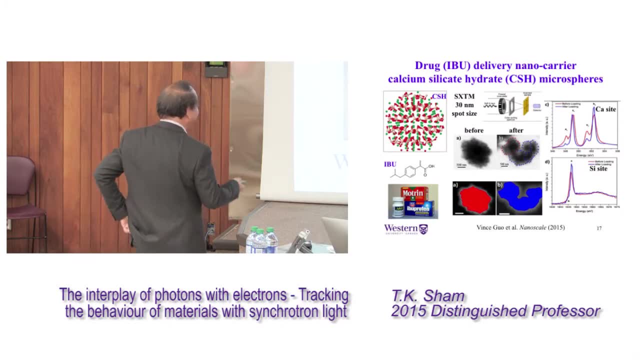 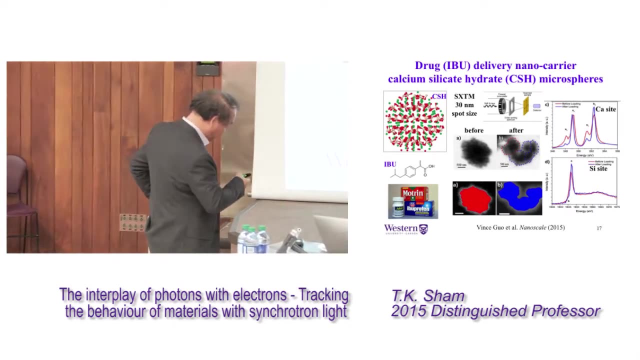 But we use the same node or material, make similar, okay, And then we can also track the chemical identity of various regions of the individual microsphere. all right, For example, we can oops. For example, we can do spectroscopy at the calcium site. 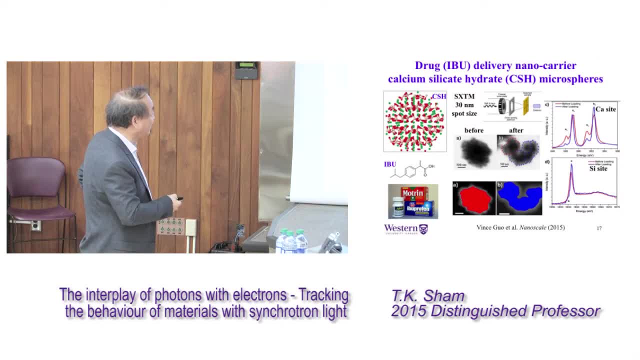 at the silicon site, and then we can compare their chemical state before and after the dose, And then we can see that the drug is loaded. So then from there we can understand how the node is and what makes it a good carrier, and so on. 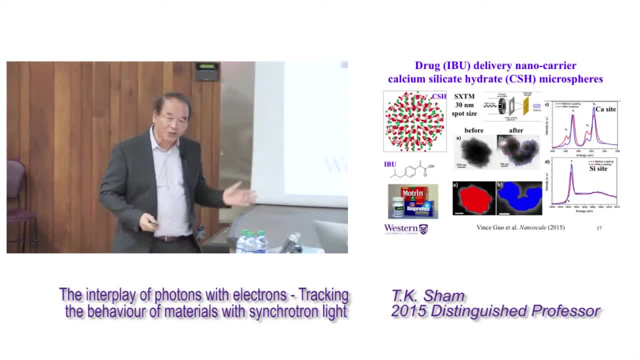 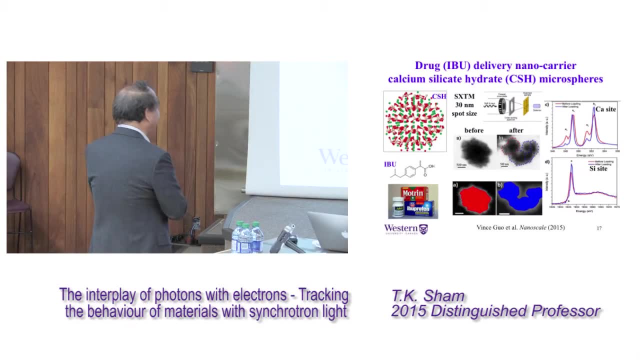 Now- and we can also because this measurement is transmission, so we can get the absolute thickness of this specimen And by doing that we will have a very good idea about the distribution If the drug loaded one way or the other, and we can get the mass of this specimen. 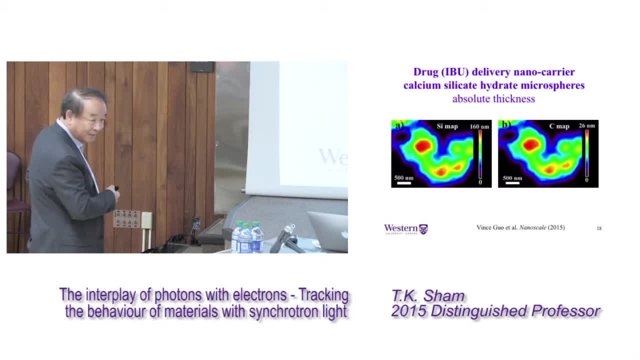 and we can get the mass of this specimen. we can get the mass of this specimen. So we can take the mass of this specimen and we can get the mass of the specimen. So this is the map of the silicon and we're tracking the silicon absorption. 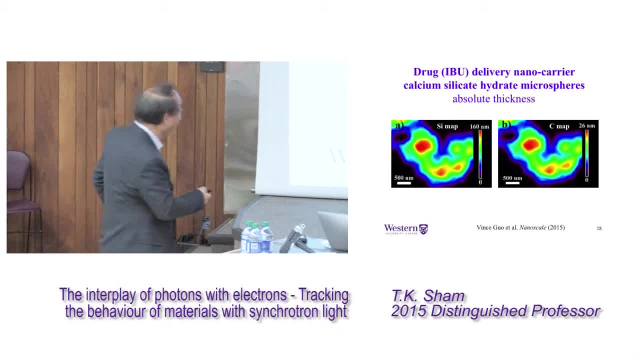 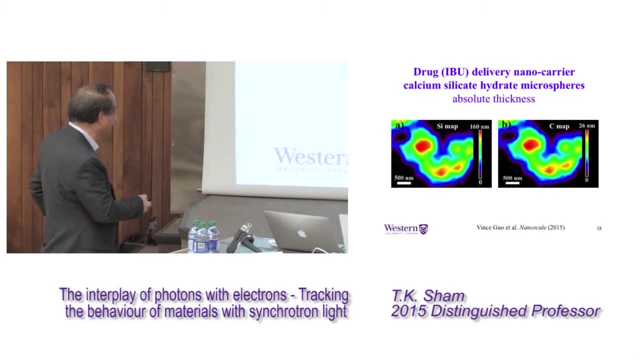 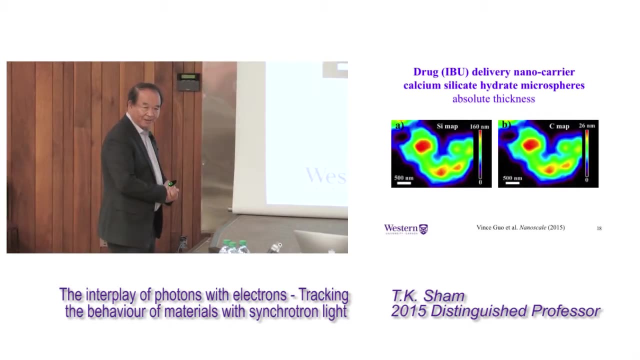 which pretty much represents the microsphere. So that gives us a distribution. the color represent the thickness. Now, this is the absolute thickness because we do the experiment in transmission. The fact that these two maps are nearly identical indicates that the drug is not very uniform. all right, 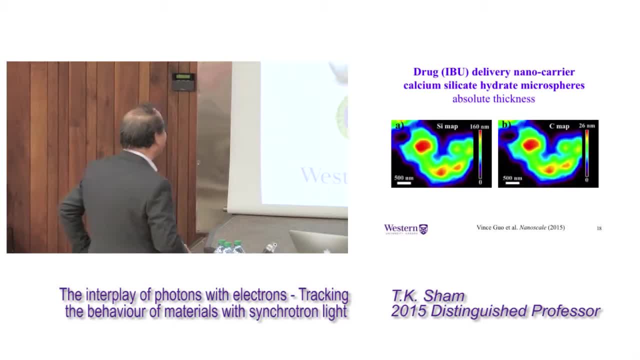 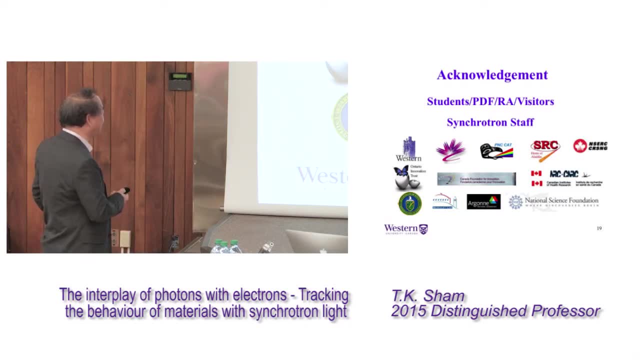 So with that I want to conclude my talk. I want to take up this opportunity to acknowledge many, many students, postdocs, research associates, visitors who have come across, come through my lab over the years, And I also want to acknowledge many, many of the Simicron. 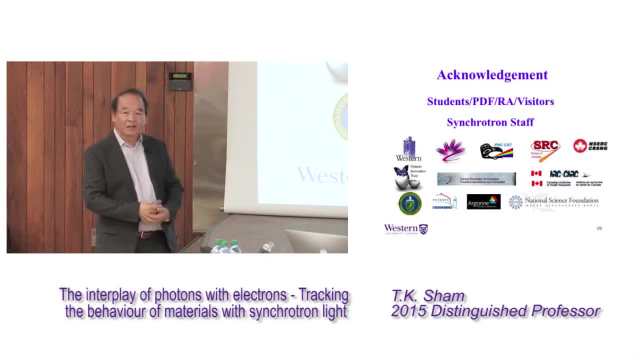 staff contributing to all of this work. I have worked at 15 different Simicrons all over the world over the years, So that's a lot of trouble And that really means understanding by the family. We've done them. This is not possible.